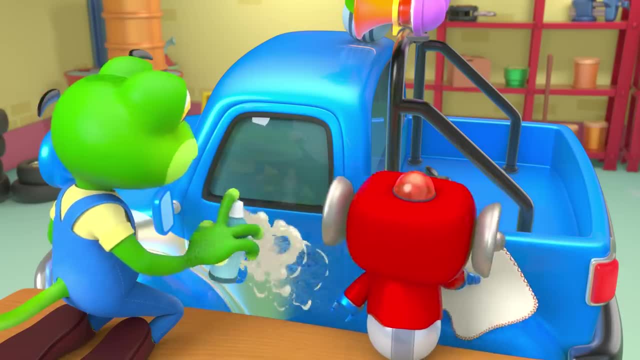 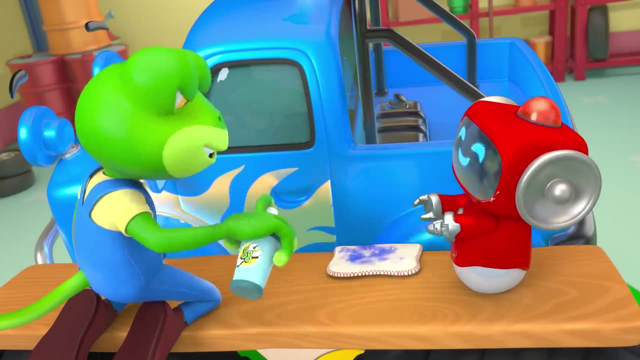 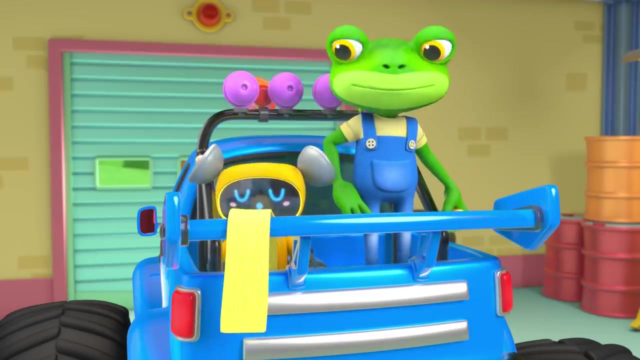 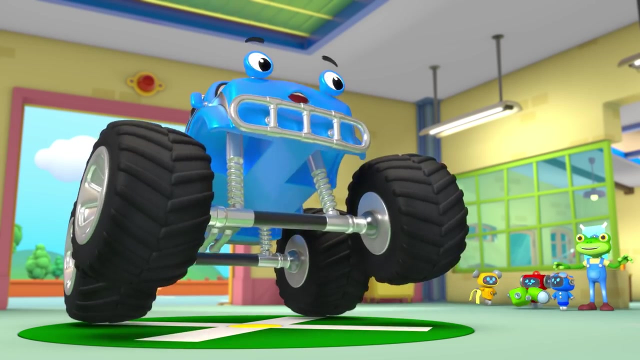 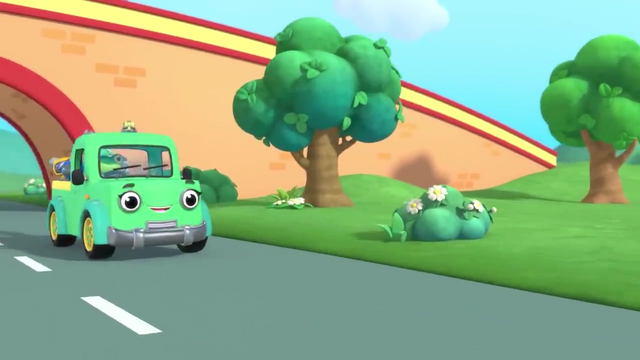 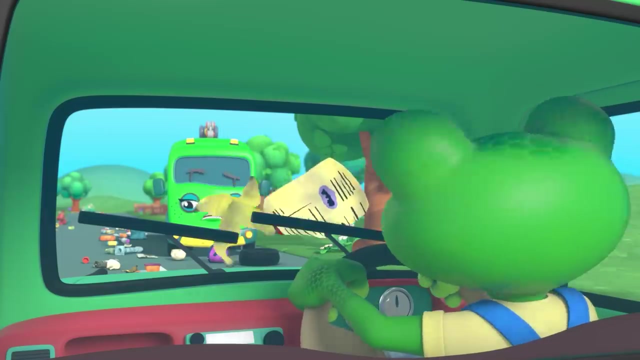 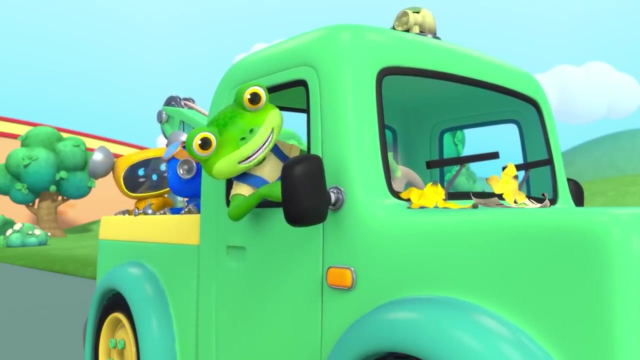 Don't worry, Max, We'll put you right. All done, Max. Is this what you wanted? Almost back at the garage Mechanicals: Whoa, Someone's dropped rubbish on the road. There's lots of it, and Mama Recycle does not look happy. 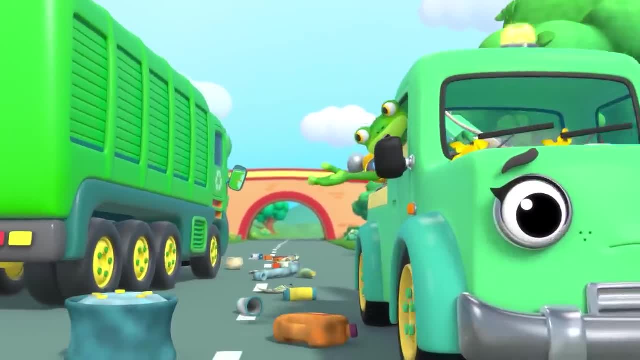 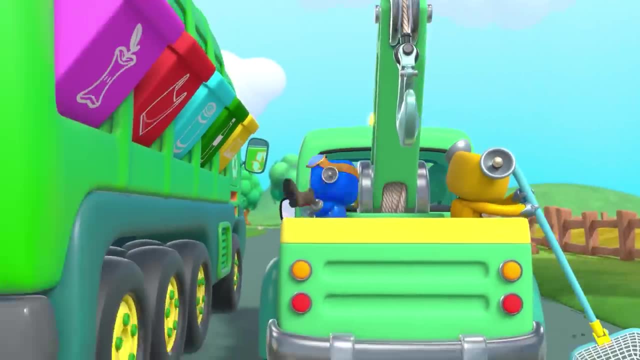 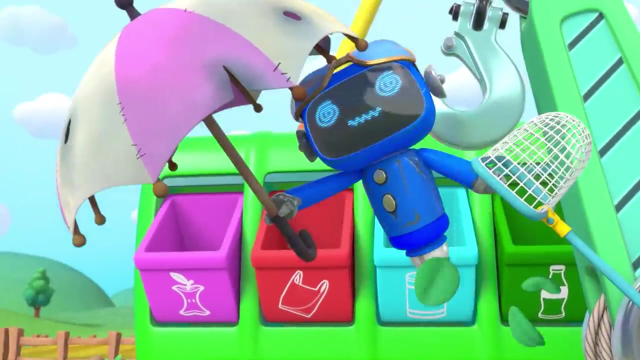 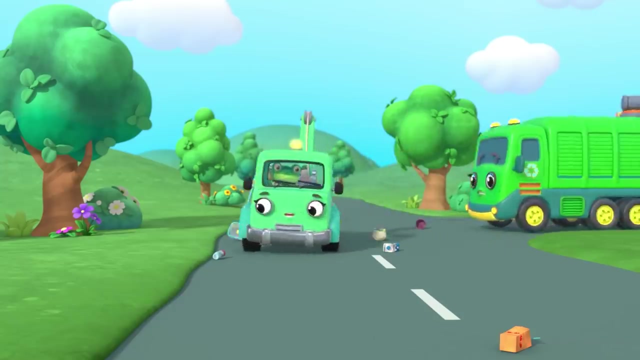 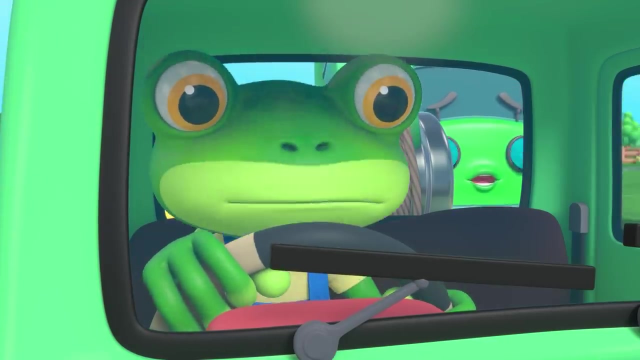 Come on, if we follow the trail we'll find out who's dropping it. Come on, let's go. Hmm, the trail goes to the left. It's Dylan the dump truck, His broken tailgate's dropping litter, But his music's so loud he doesn't notice. 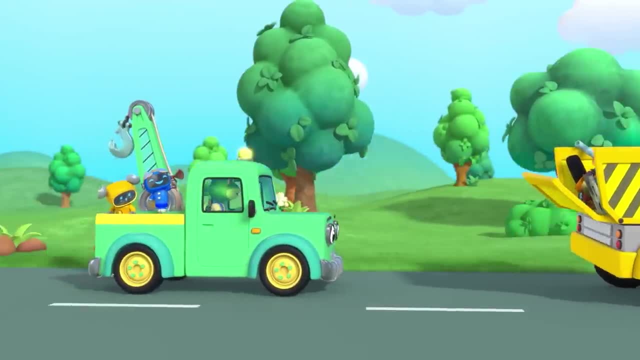 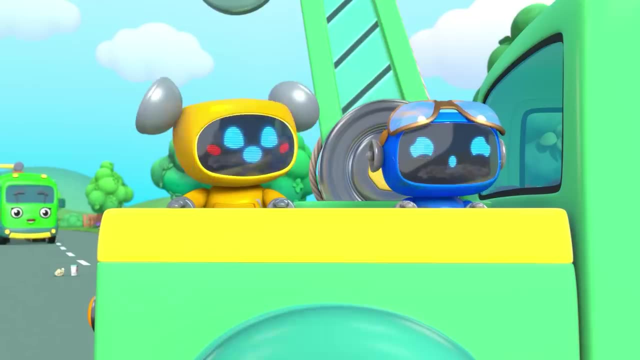 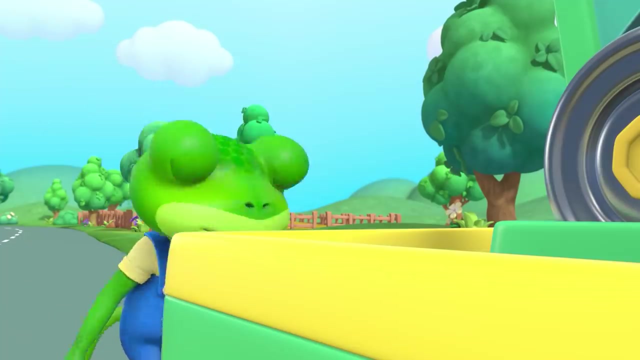 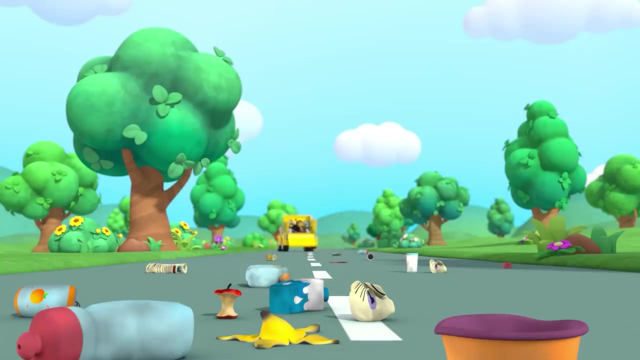 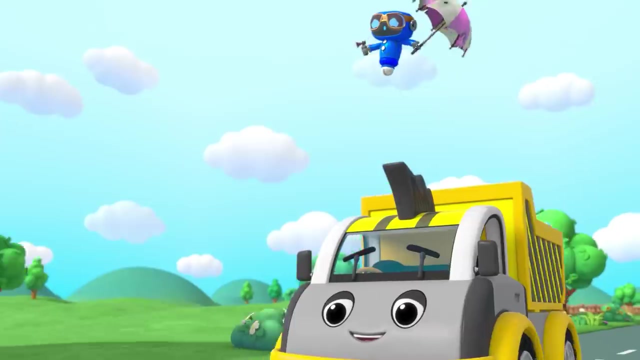 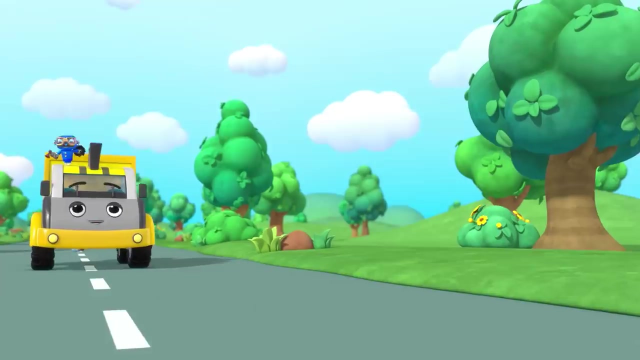 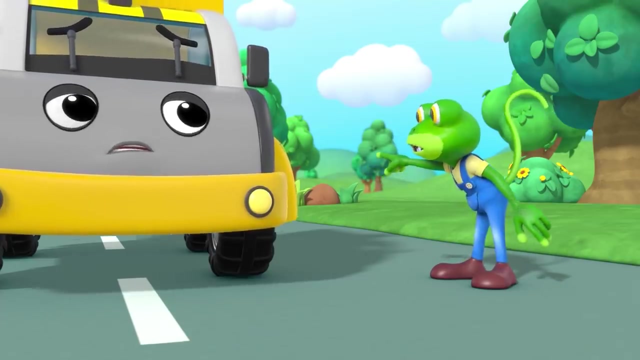 Oh, Mechanicals, we've got to turn down Dylan's music. Let's recycle and save the day Using things we've thrown away. Andación, Dylan, Dylan, Your tailgate's broken, But don't worry, I'll fix it. 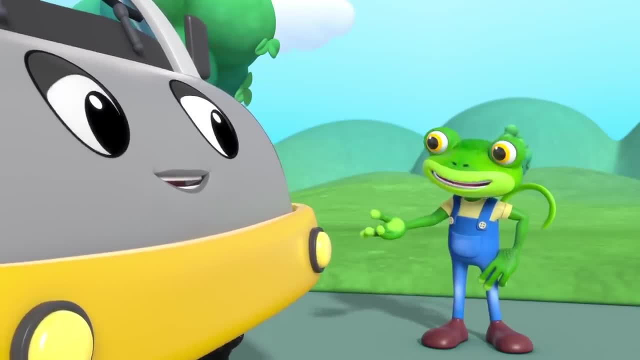 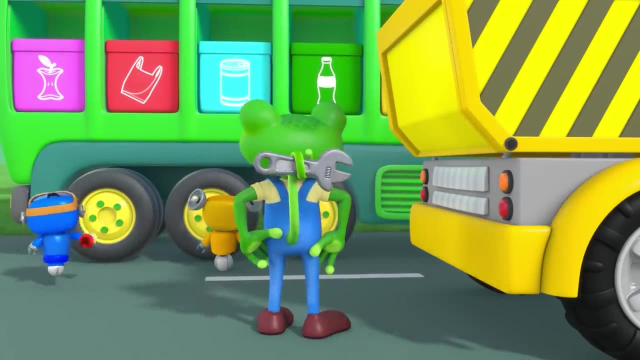 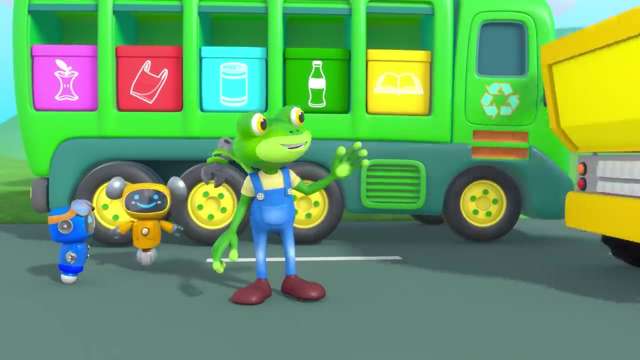 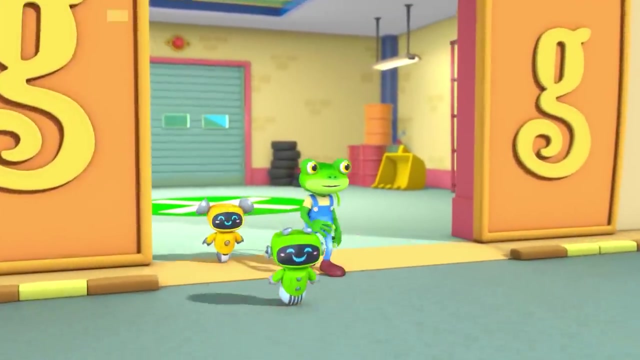 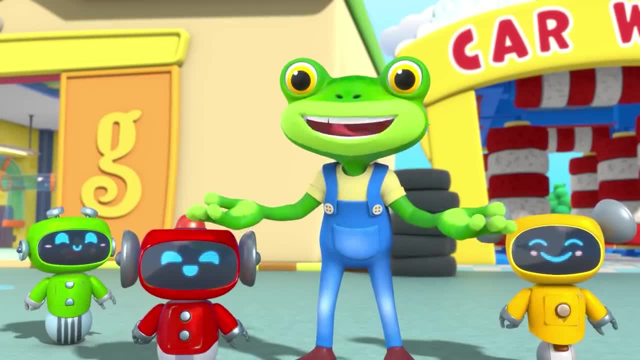 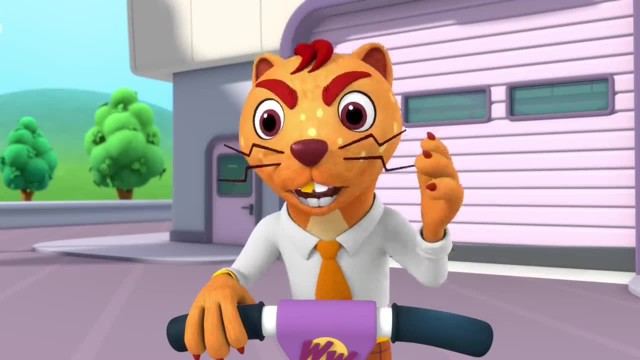 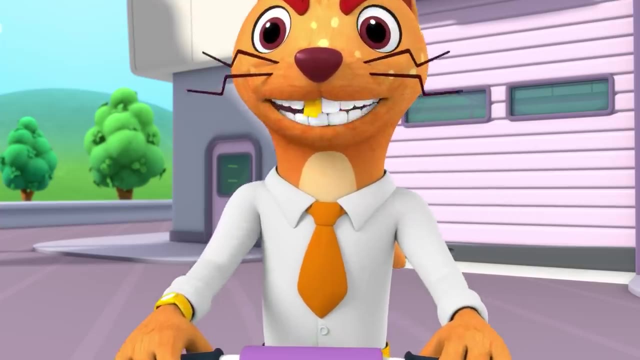 Oh, dear, Come on in and we'll get you nice and clean in our car wash. You call that a car wash. You're no match for a weasel wash. I can clean any vehicle better than you. Up to the challenge, Gecko. 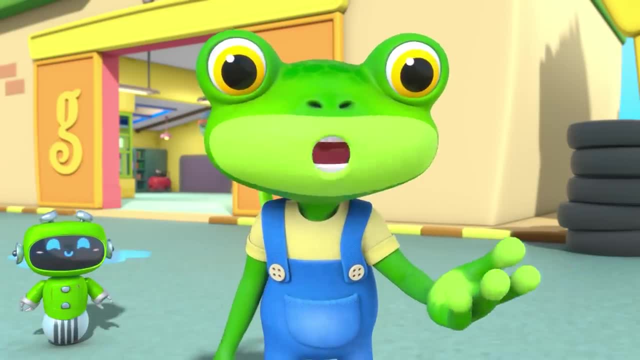 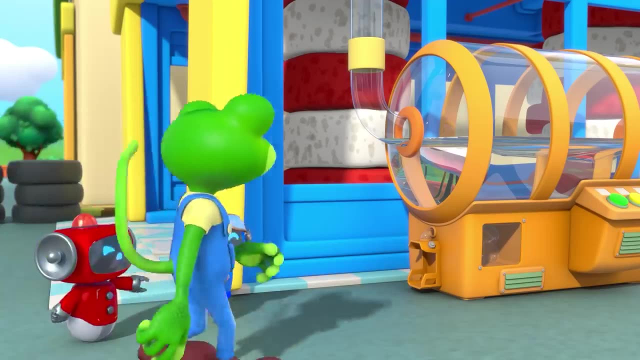 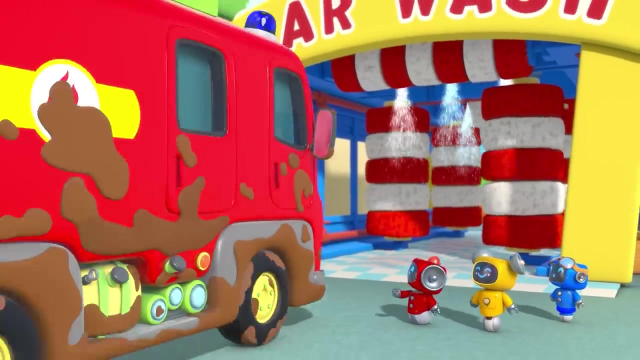 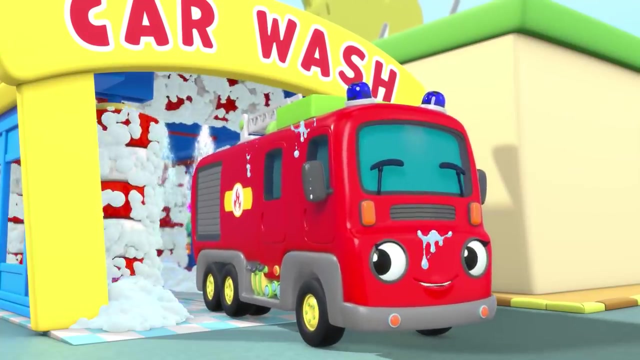 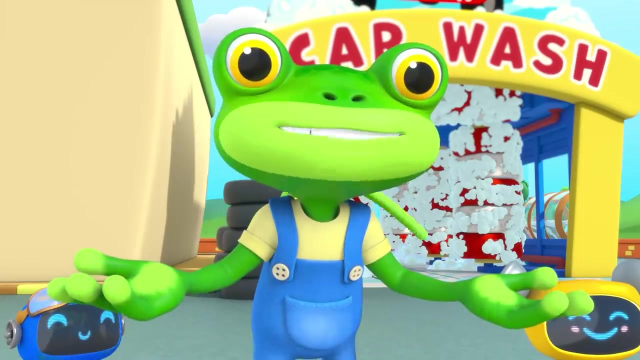 Sure, Sounds like fun. How about we take Fiona and you take Bobby. Ready Mechanicals, Ready Mechanicals, Ready to go? Fiona, Your turn, Mr Weasel. Good luck, I don't need luck to clean this muck. 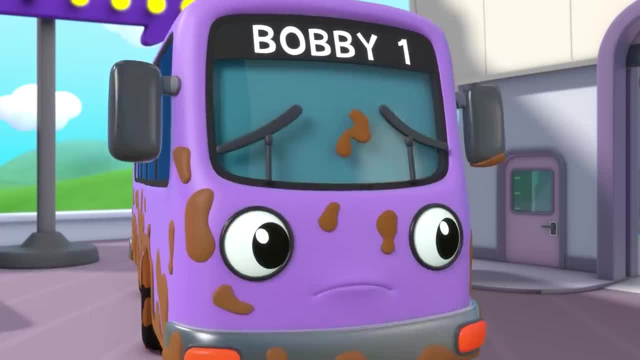 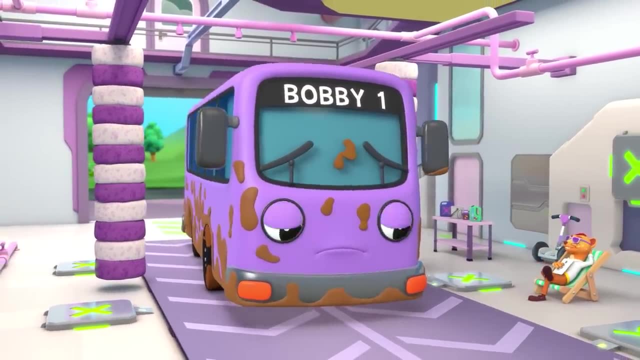 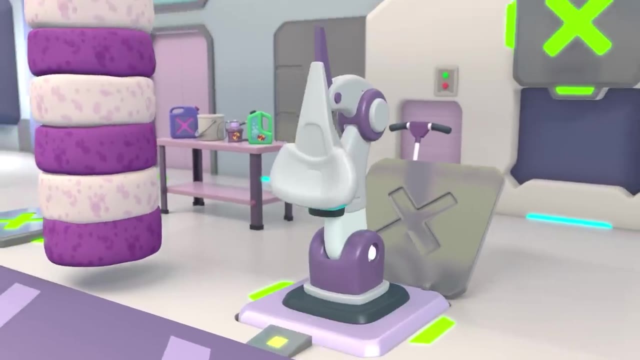 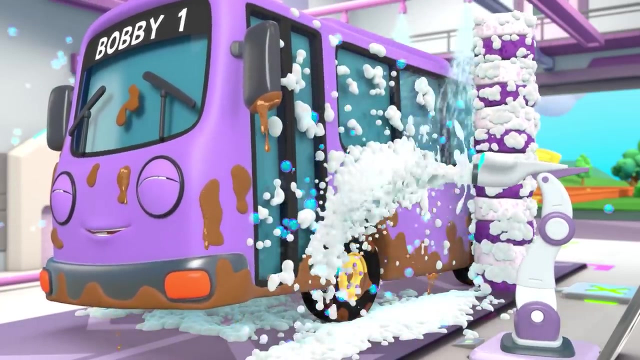 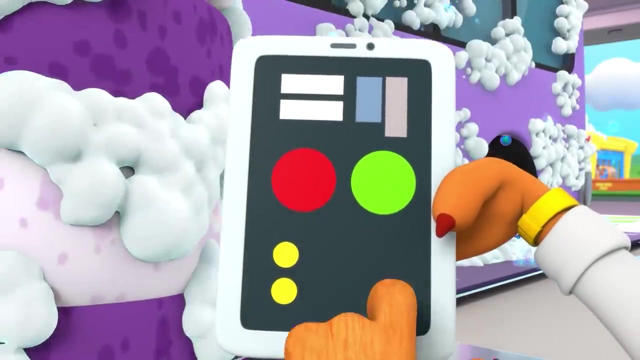 In you go, Billy Gary. Haha, More power, I think. Oh, That's the VB tune, I guess not. OK, Got it. OK, Got it. Can we clean it now? Good, Aha, ha, Right-o. 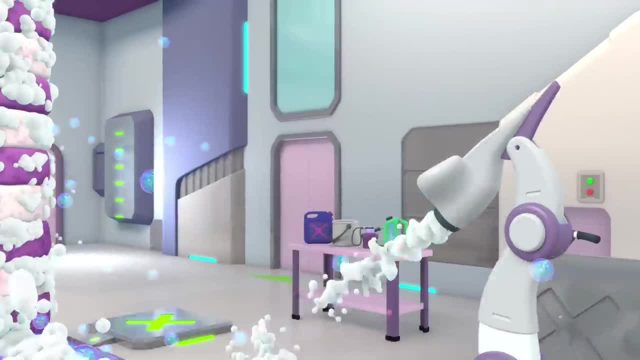 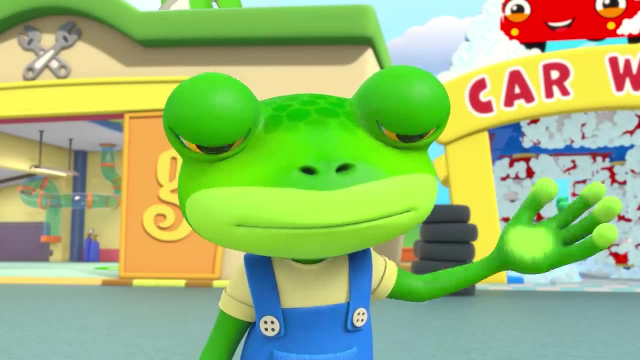 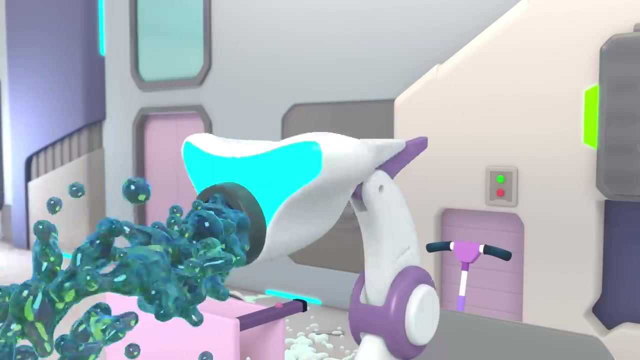 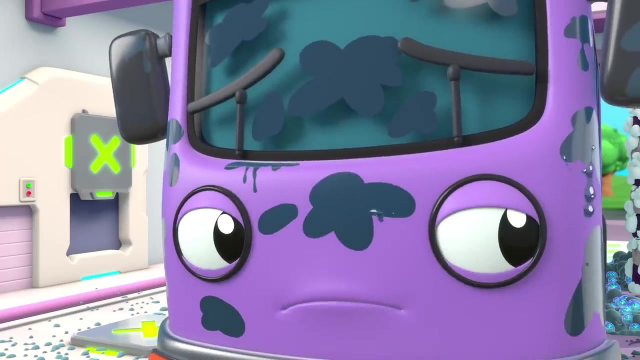 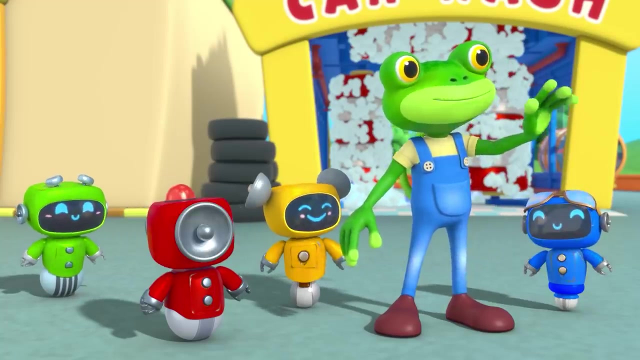 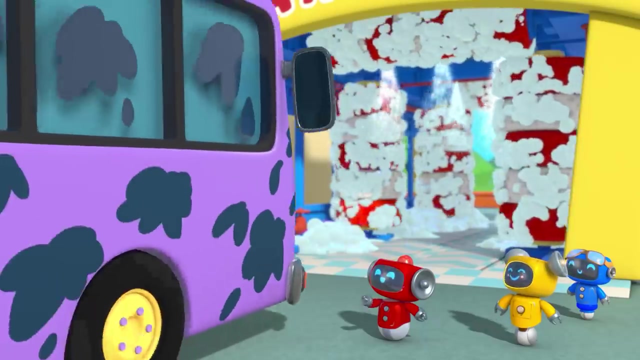 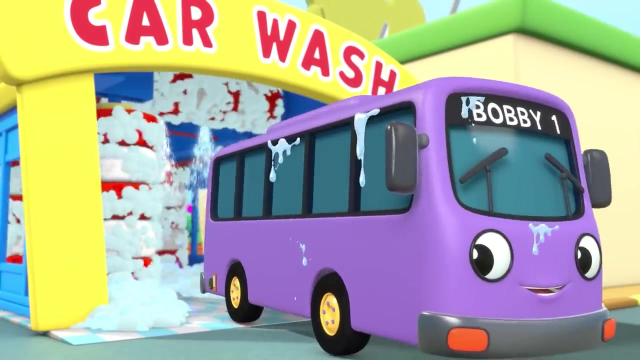 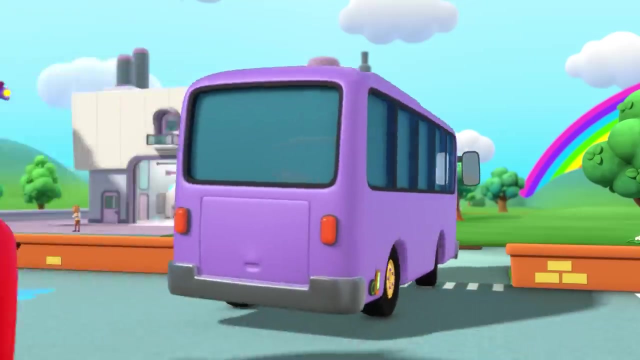 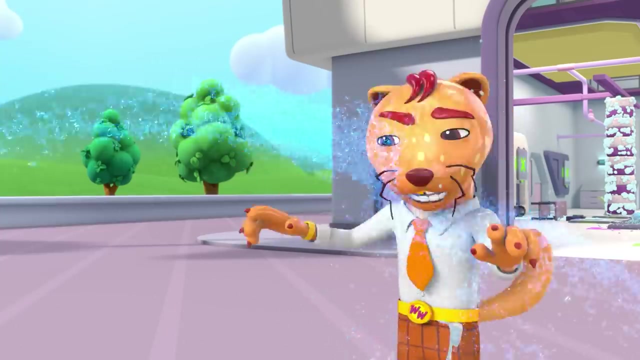 That's a good one, Moses. I'm going to clean this bopper with some oldgettes. Oh Dear, that doesn't sound right. Nevermind, Bobby, come on over and we'll do our best to get you clean, Sparkling clean. Come on in, Mr Weasel, We'll get you dry. No, thank you. 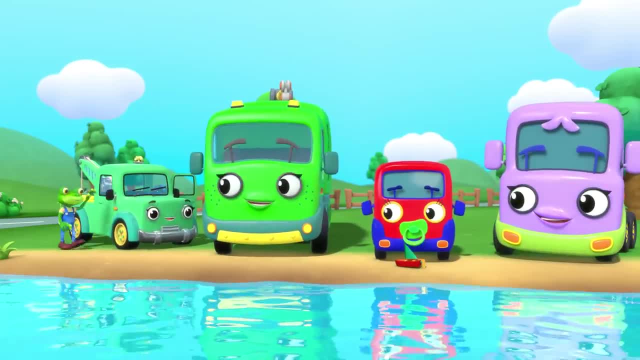 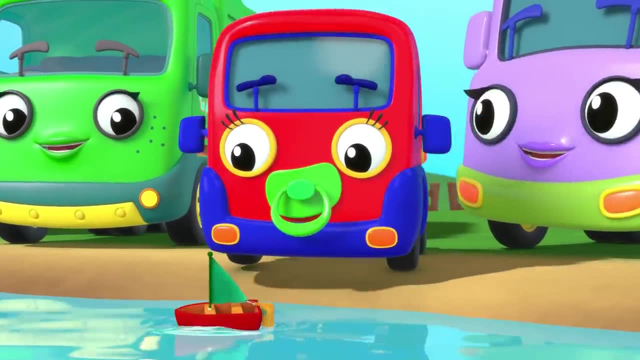 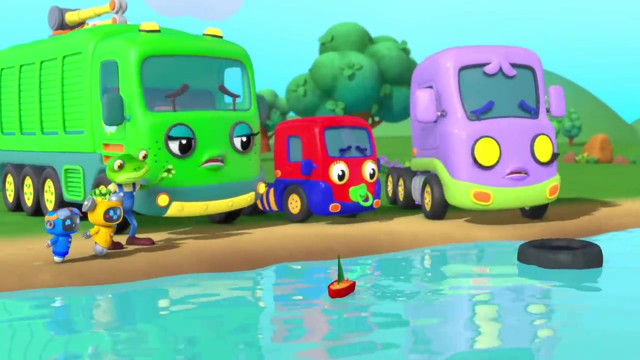 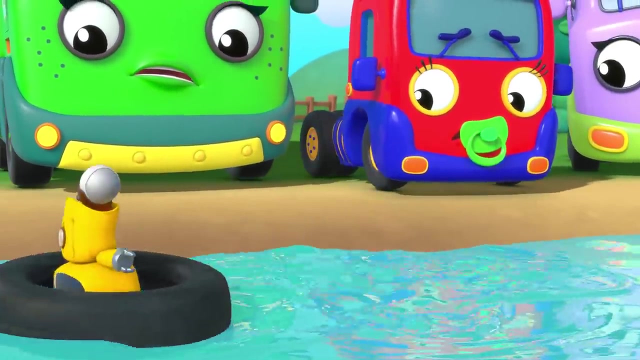 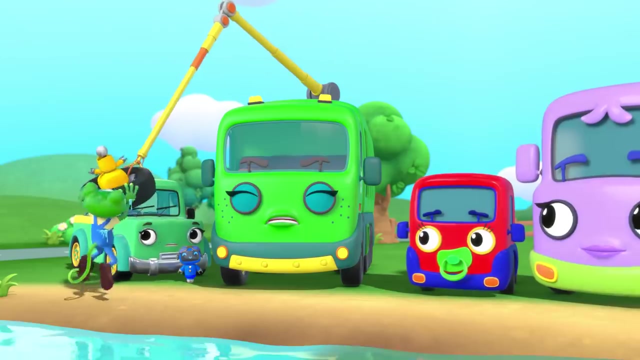 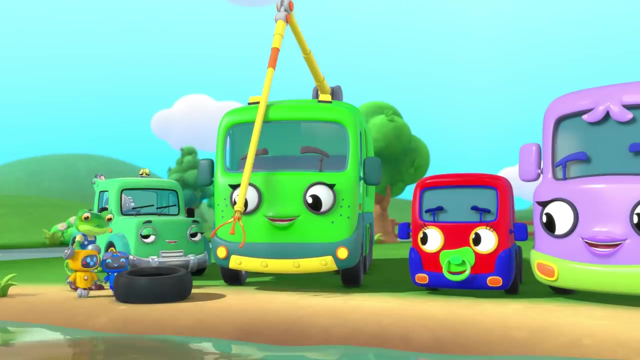 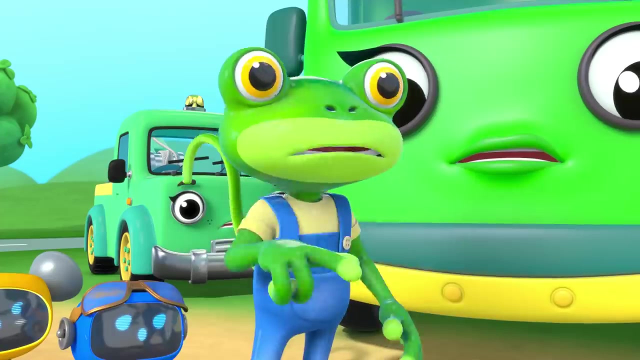 Mechanicals. it's the truck family. Good morning everyone. Oh, that's a nice boat. You have their baby truck. Oh No, attire, it's heading right towards baby. Oh Thanks, mama, now we can recycle that old tire. They must be coming from somewhere. upriver, let's go. 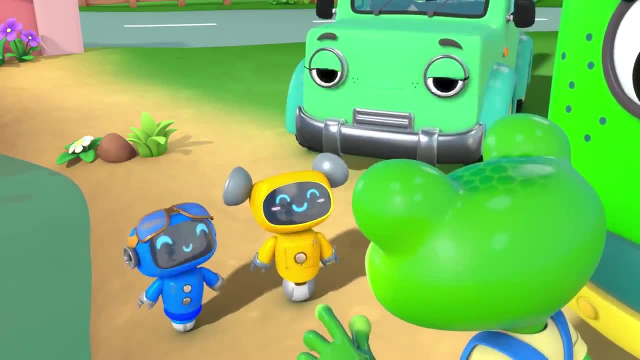 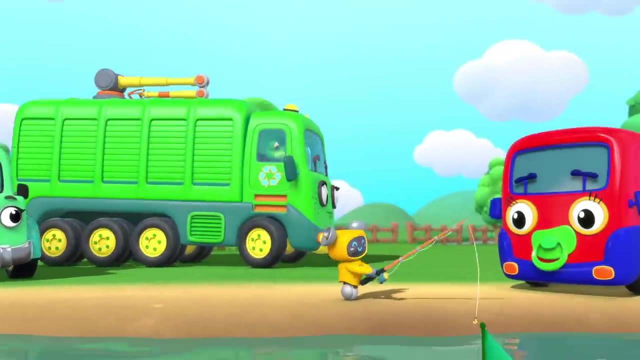 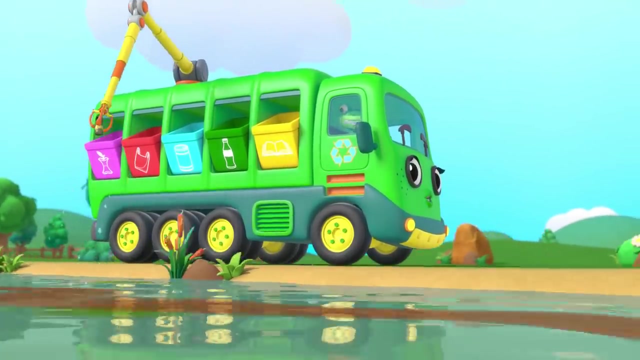 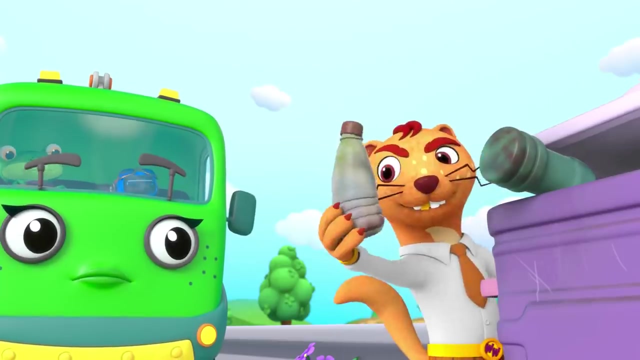 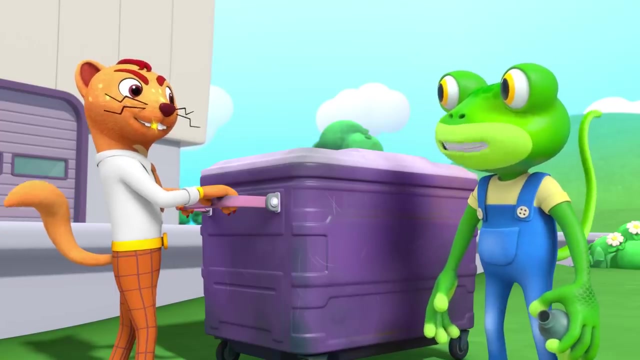 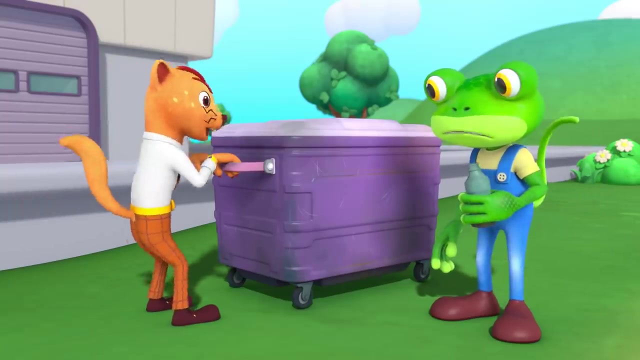 Stay here. yellow, protect the boat. More rubbish there. where could it be coming from? Mr Weasel, what are you doing? Oh, gecko, I was trying to get rid of all my rubbish. Oh, The brakes are stuck. You shouldn't throw rubbish in the river, Mr Weasel. 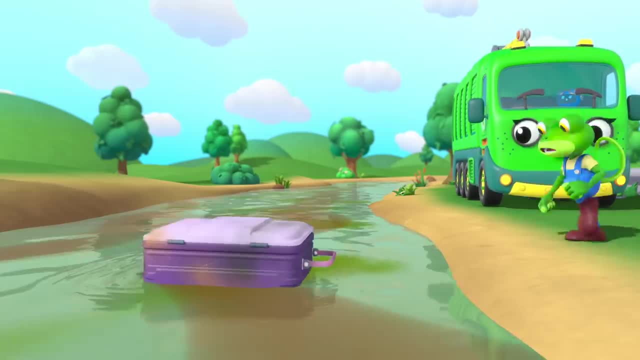 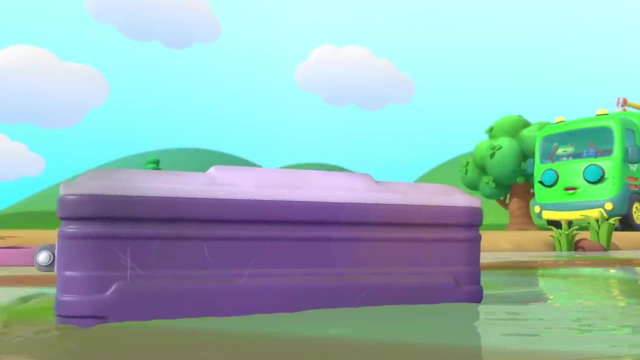 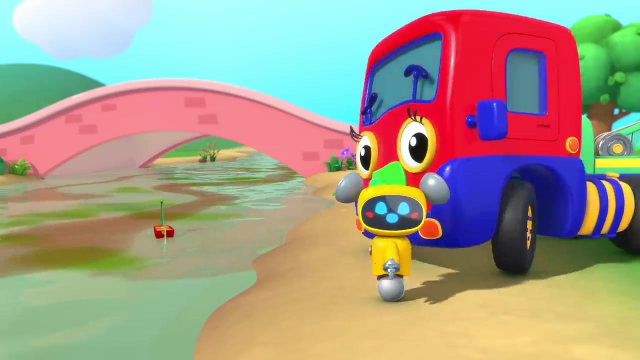 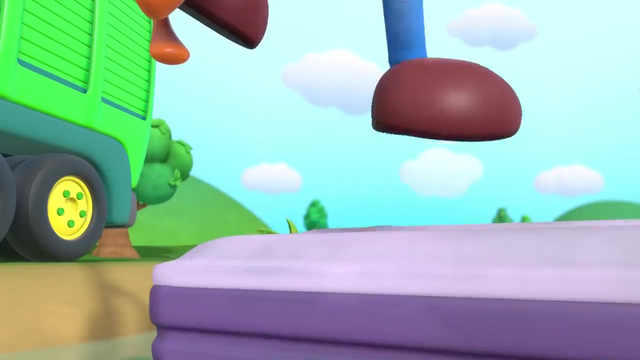 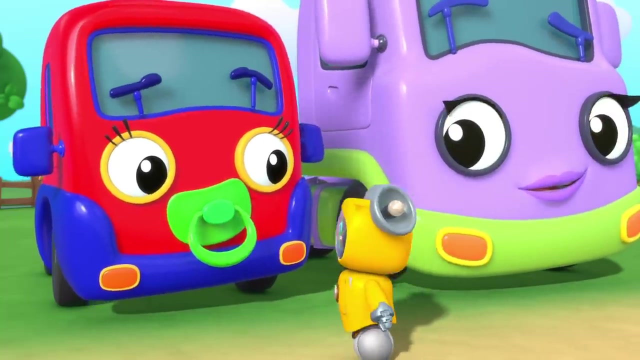 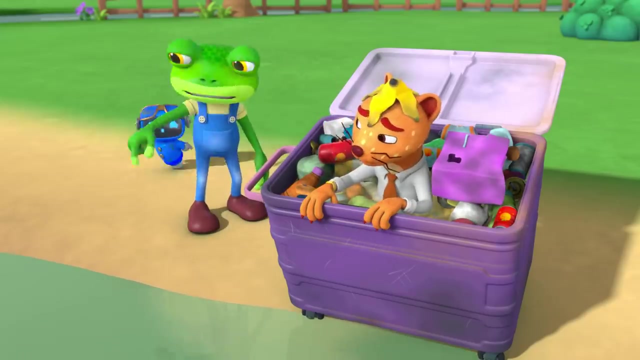 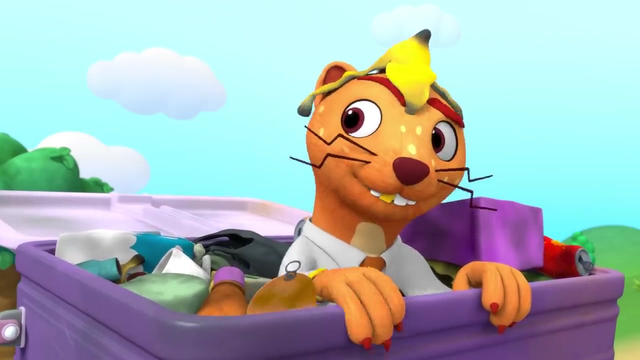 Oh No, he's heading right towards baby truck and her boat. Oh Oh, You shouldn't throw rubbish in the river, Mr Weasel. it makes the river dirty. you almost wrecked baby trucks, toy boat, a boat. I I've not played with a boat since I was a young weasel. 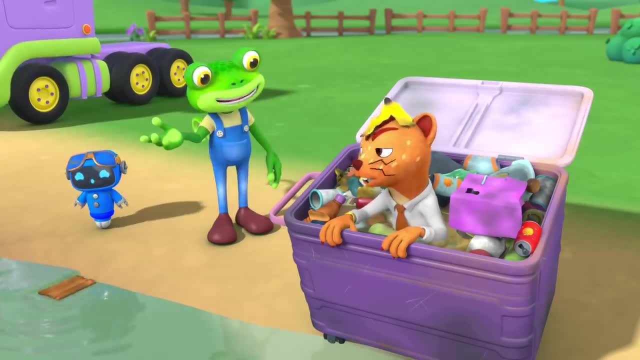 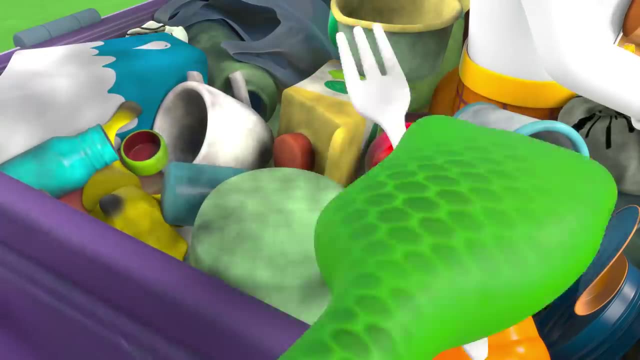 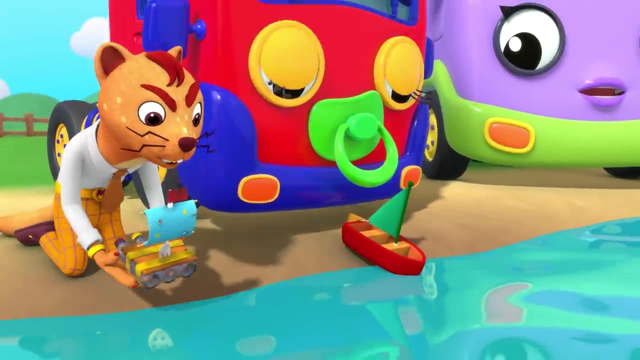 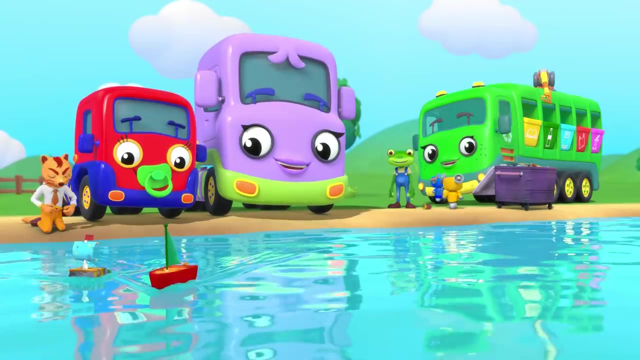 I have an idea. Rubbish can be recycled. instead, Make shiny new things from old things. Let me show you Who are. Hoist the anchor: Look out, Here comes the good ship Weasel. This is so much fun. 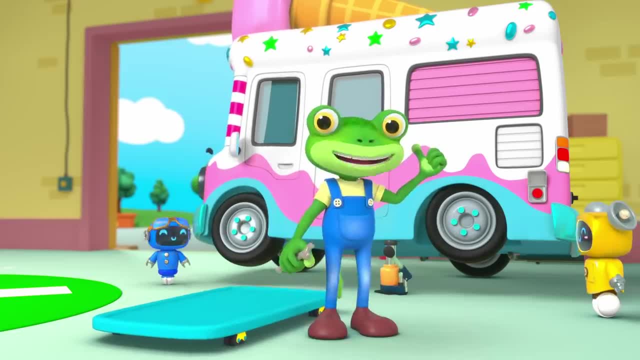 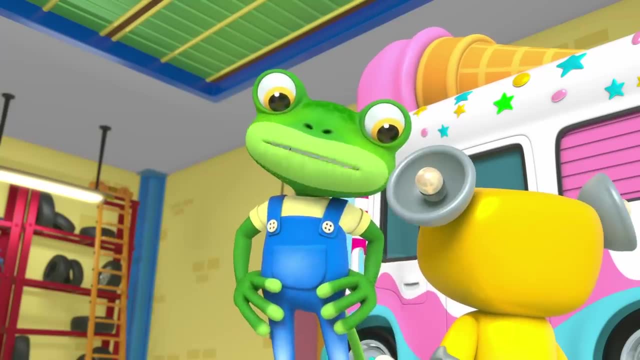 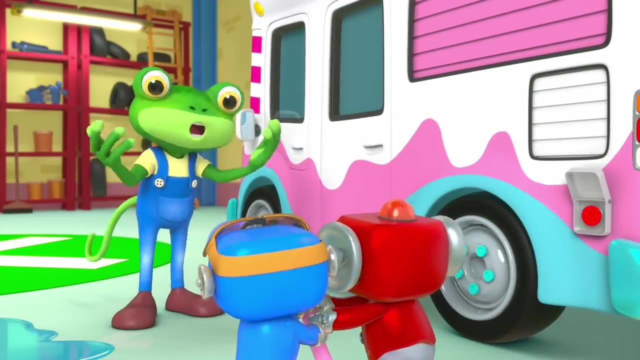 Oh, hey, there everyone. Vicky, the ice cream truck, is in for her repairs. We're just doing a few finishing touches. Thanks, Yellow. Could I please have a screwdriver? Careful Mechanicals. That pipe is full of ice, cold air. 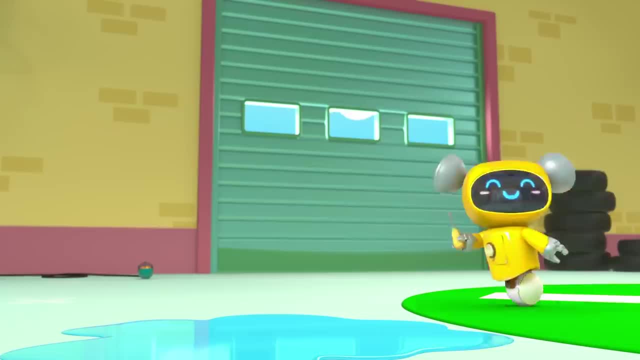 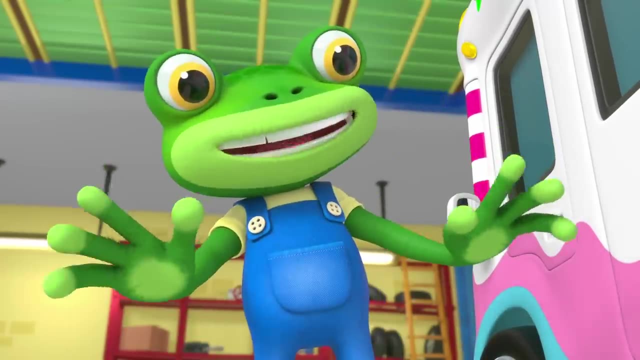 It's how Vicky freezes her ice cream. Where's the other ice cream truck? We've got to get her back. Drink some. Oh no, I don't like ice cold water. Here comes the Vicky the ice cream truck. 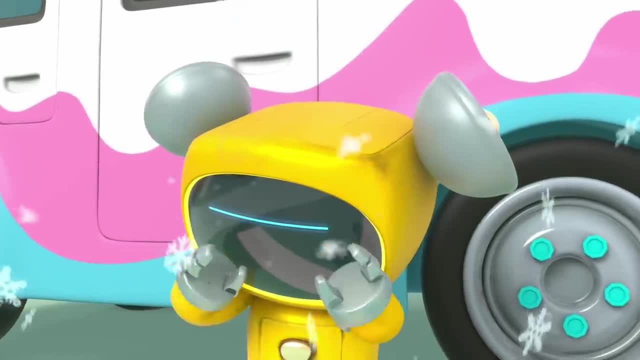 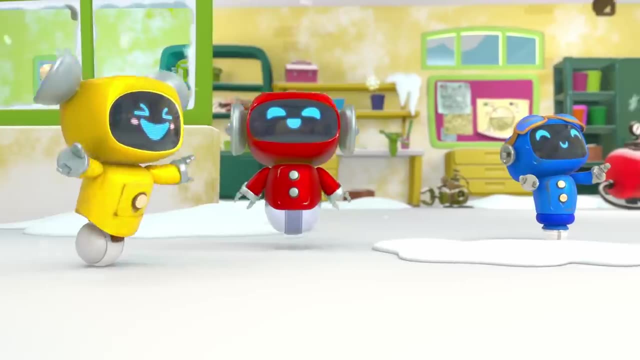 You've got all the ice cold water- Yellow. don't touch that button. An ice cold water is weird, huh? You know that you can't catch a cold with ice cold water- Yellow, Don't touch that button. Mix and mix. 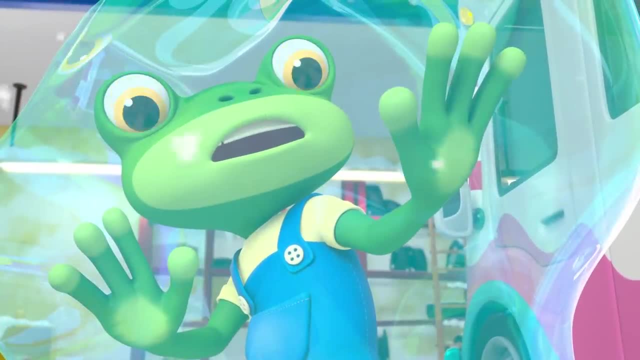 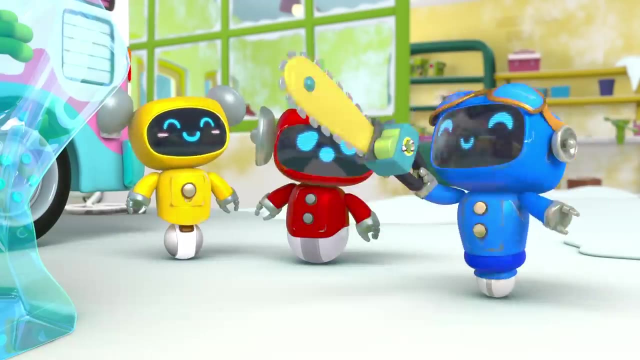 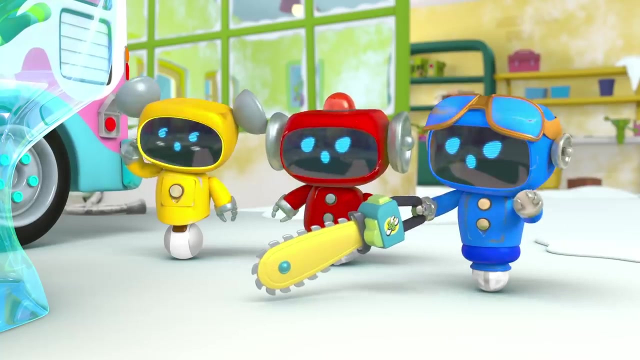 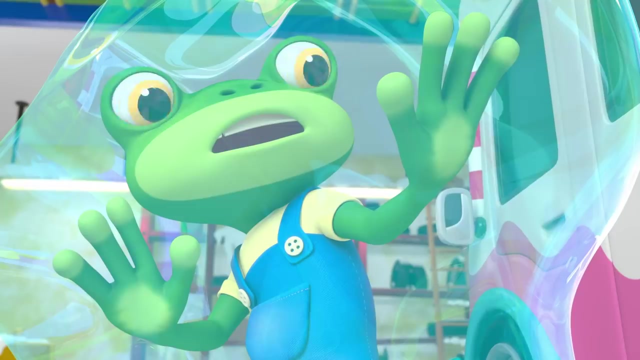 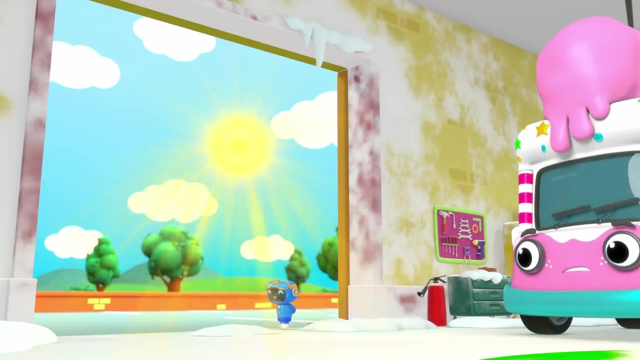 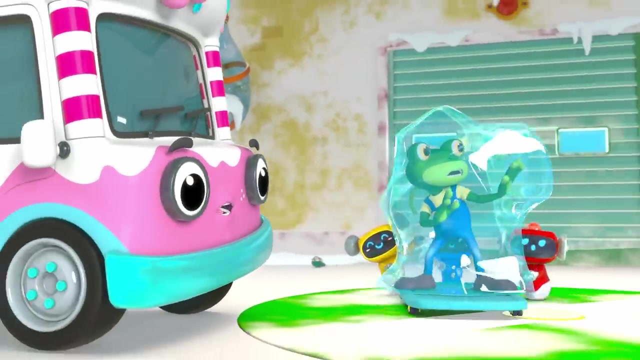 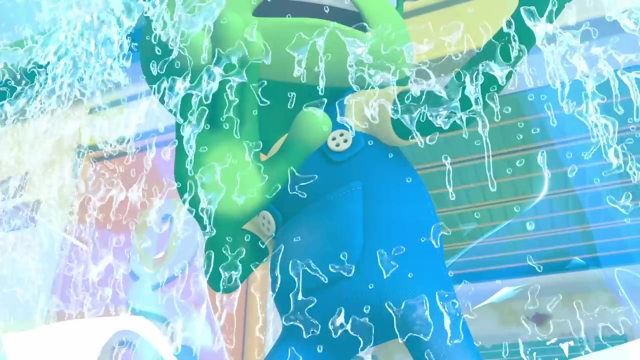 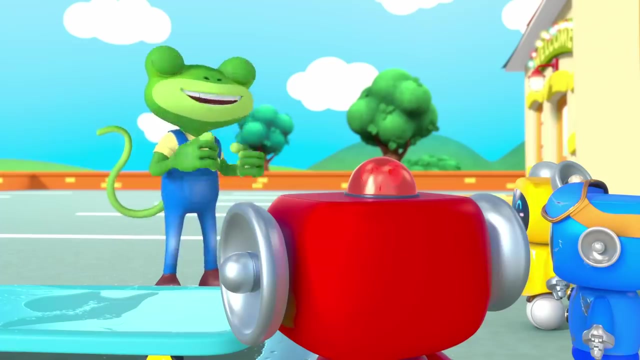 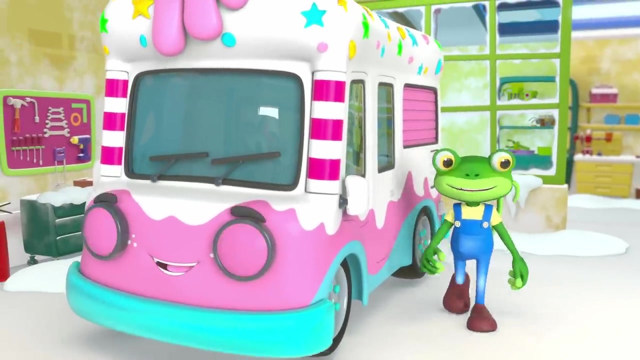 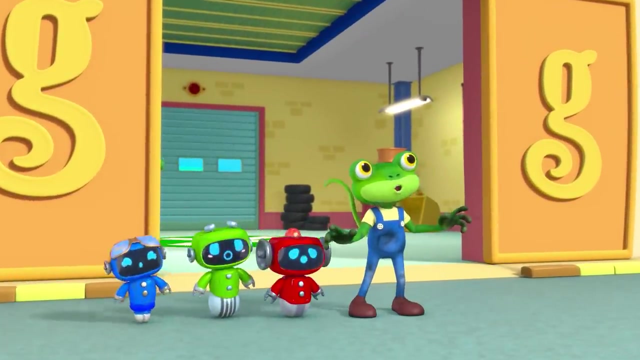 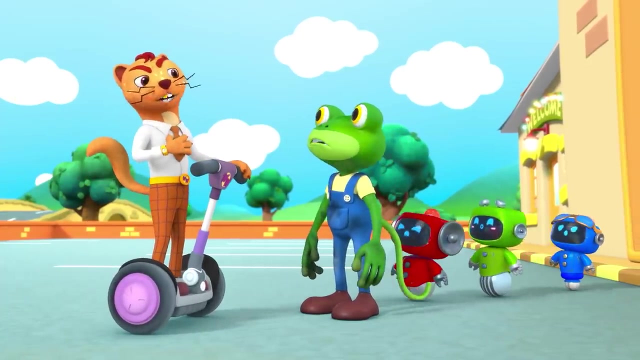 Oh, jelly beans, Shush yellow, Don't touch that button. Oh, no, Phew, thanks, Mechanicals, You saved me. Now let's finish fixing Vicky. Come on, Mechanicals, we have Fiona Firetruck in today. I'm Wilbur T Weasel, owner of Weasel's Wheels. 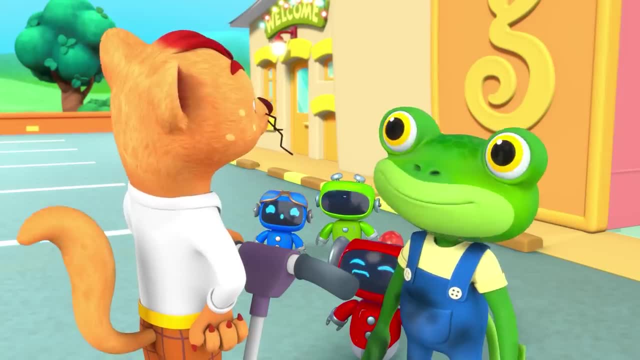 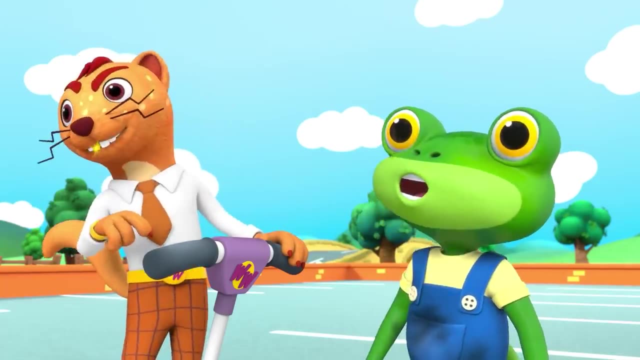 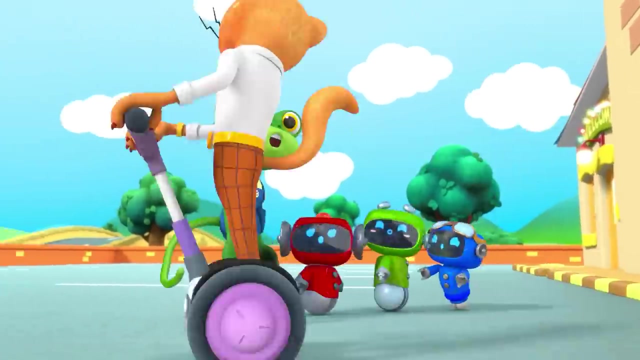 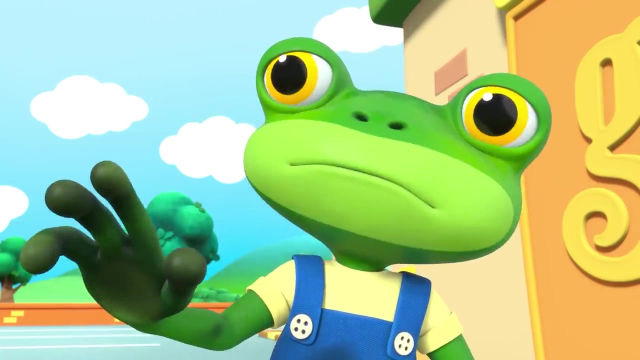 Fully automated to fix things fast. Hello, Mr Weasel, I'm Gekko. Oh, here's my first customer. Every job is quickly done. So Weasel's Wheels is ready to go. Weasel's Wheels is number one. See you, Frog Er, the name's Gekko. 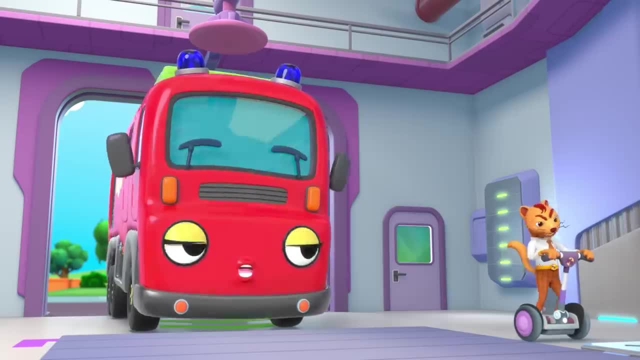 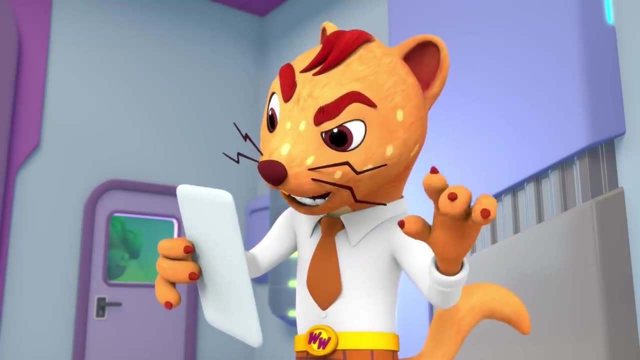 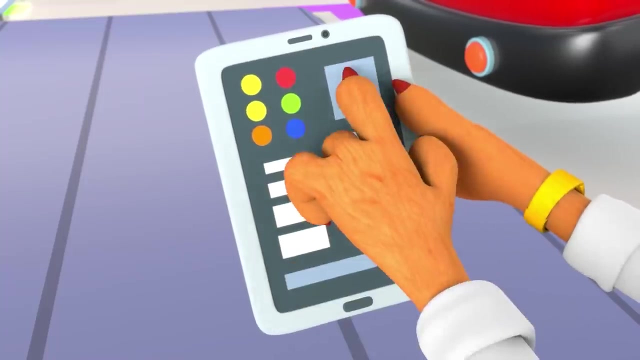 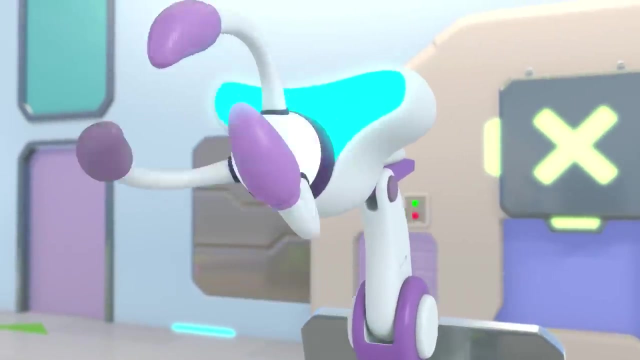 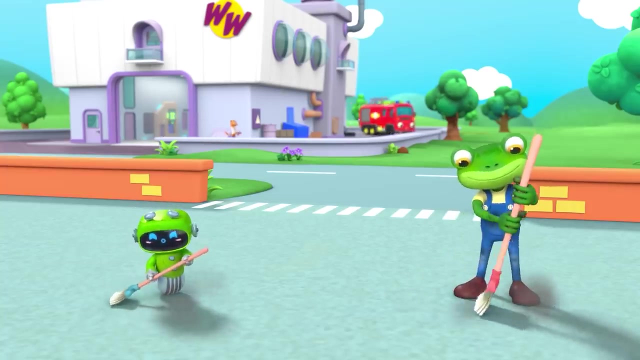 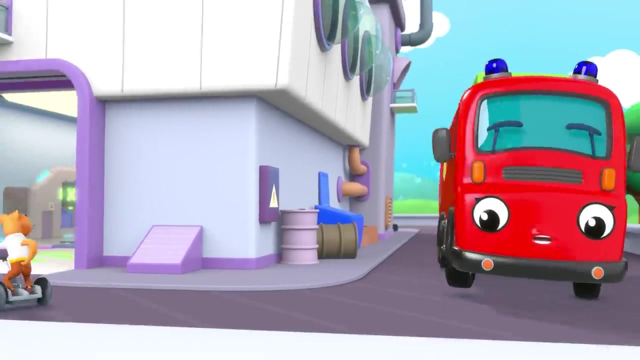 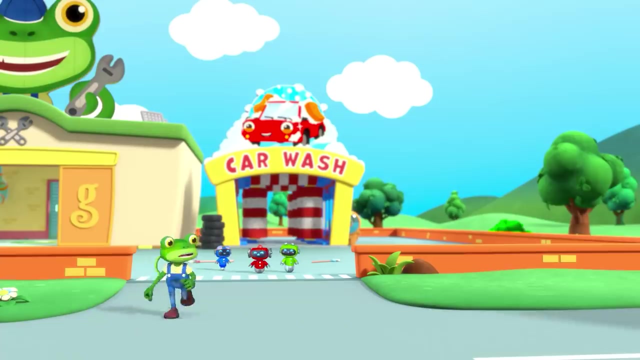 OK, Floella won't take long. Hmm, I'm not too sure which button starts the service. Oh, pressing them all should do the trick. Come again, Felicity. That was quick. Oh dear, she doesn't look good. Come in, Fiona, let's have a look. 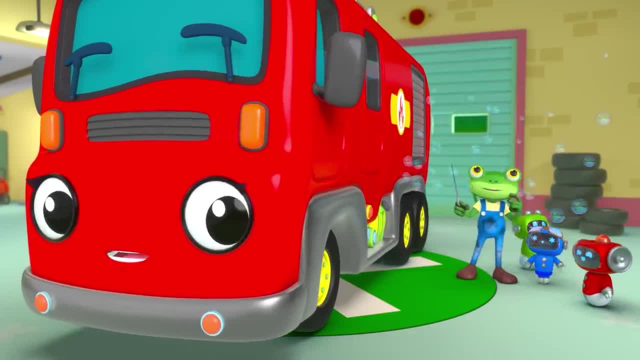 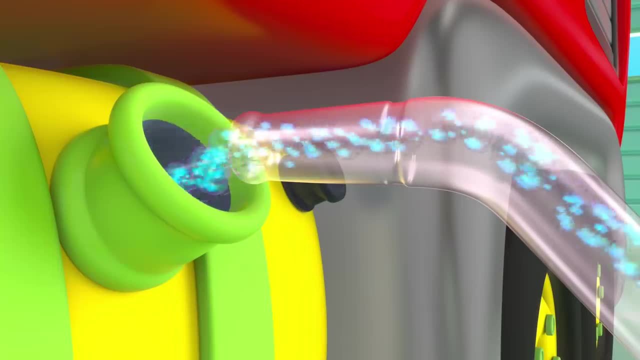 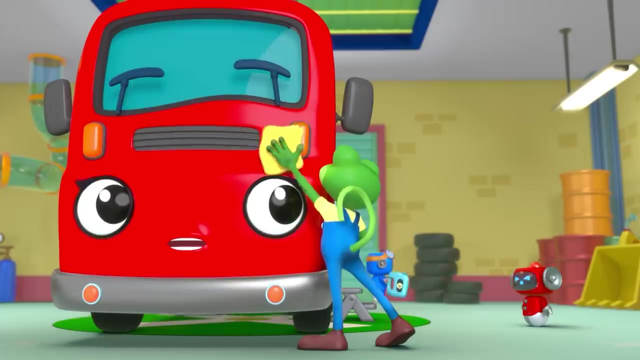 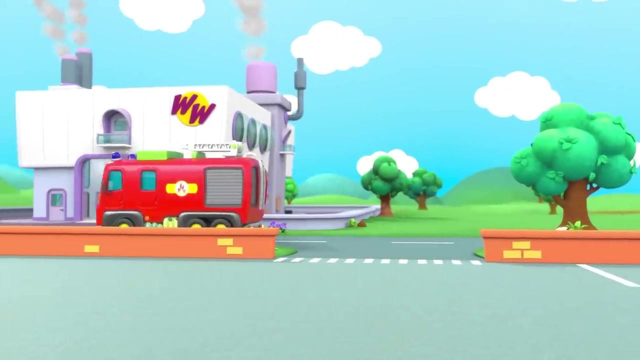 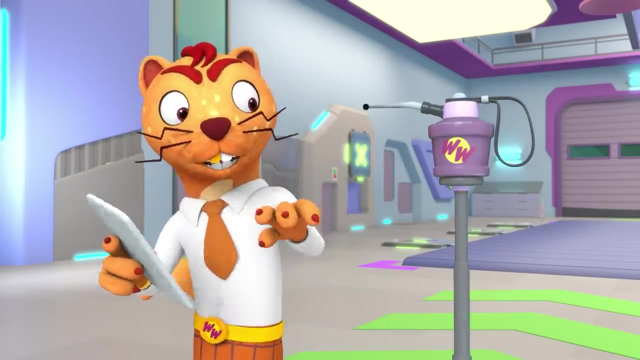 That's the problem. Weasel was in such a rush to get things done That he put soap in your tank instead of oil. We fixed the problem properly. Now Fiona's running bubble free. Hmm, I'm sure I pressed the right button. Oh, it's not working. 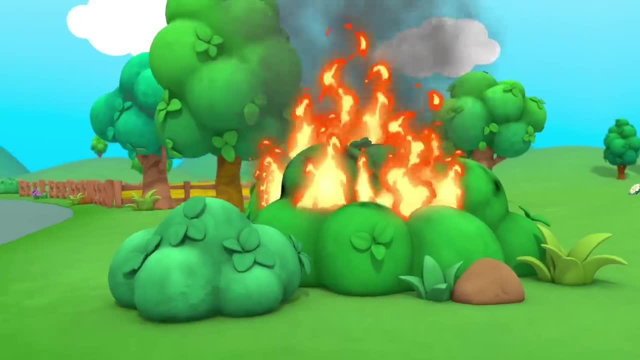 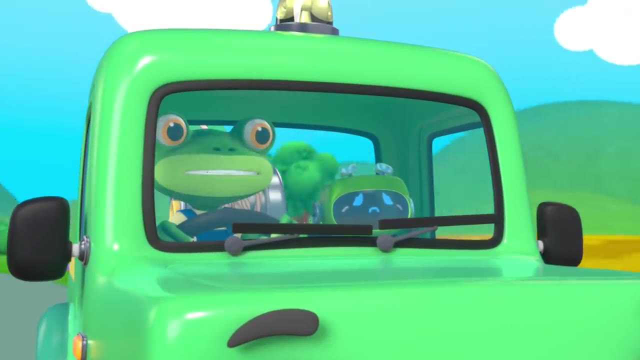 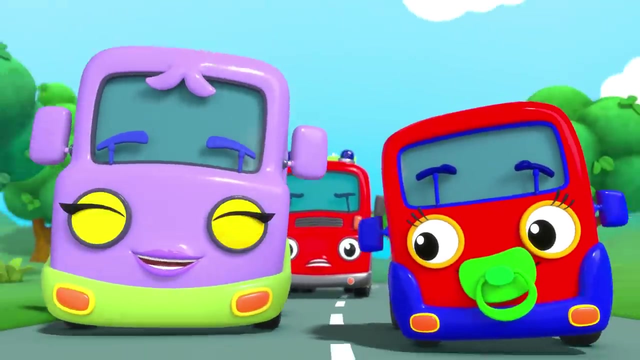 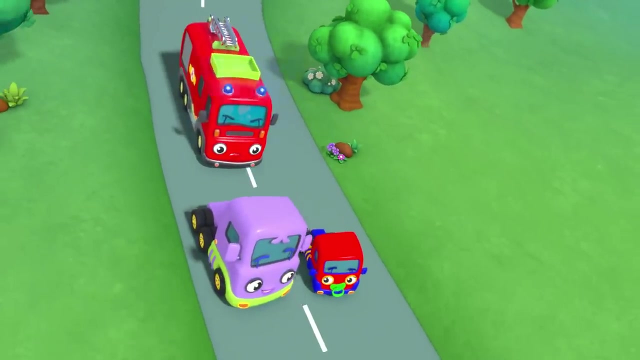 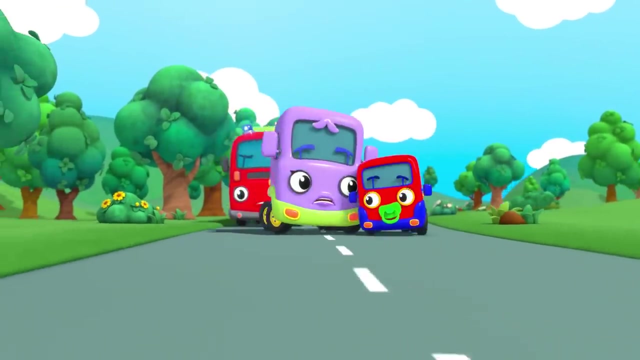 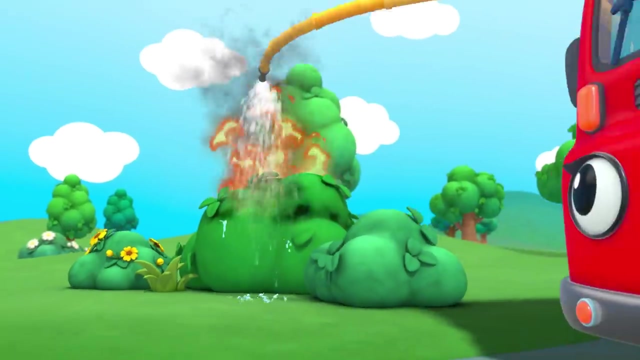 Yuck Oops. You're right, Green, there's a fire. It looks like Fiona Fire Truck is on her way. Oh no, Mummy and Baby Truck are having a play race. They're brumming too loud to hear Fiona's siren. Fiona, it's time we fitted you with a louder siren. 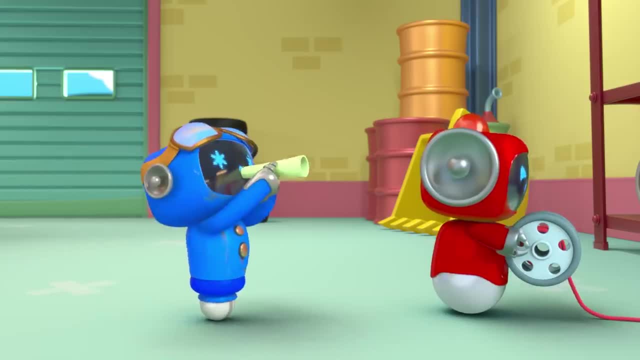 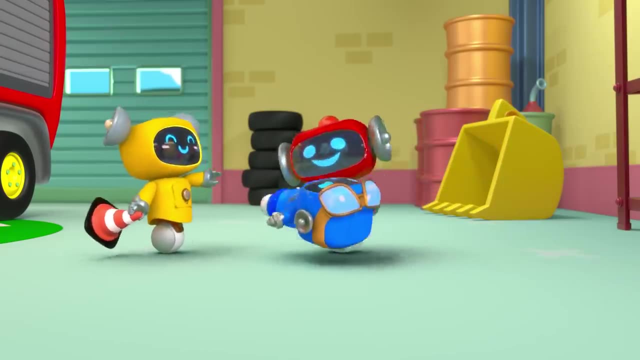 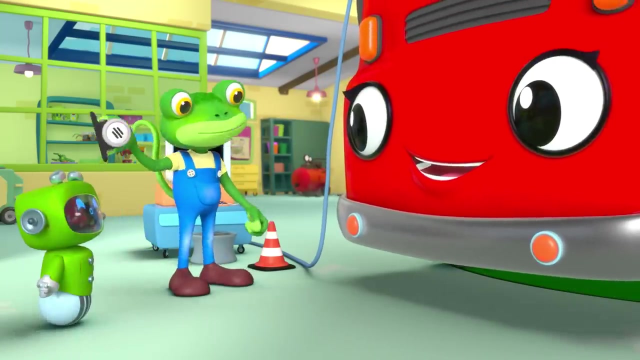 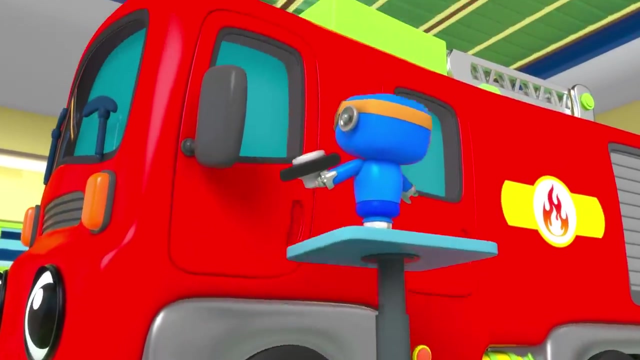 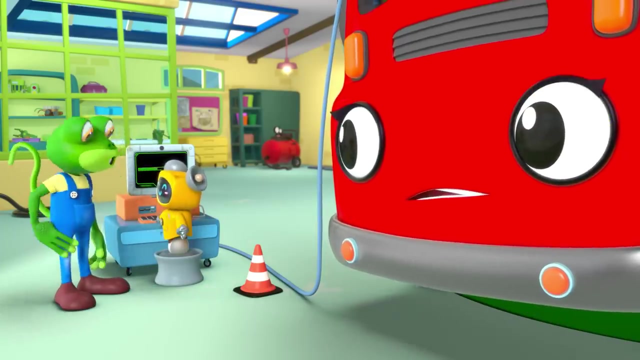 Come on, Mechanicals time to fit Fiona's new siren. I'm going to fit you into the siren. I'm going to fit you into the siren. I'm going to fit you into the siren. That's it. we need a nice loud neenaw sound. 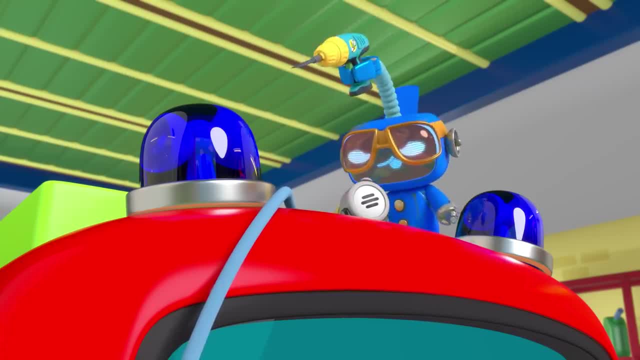 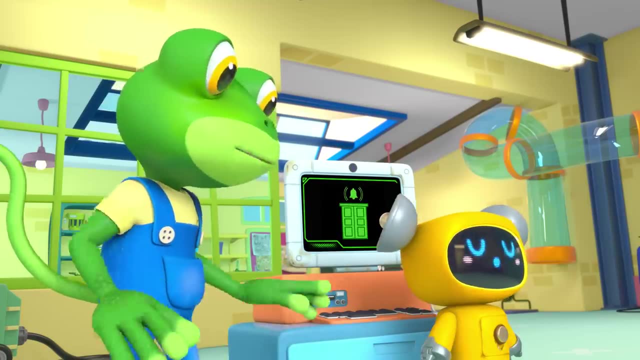 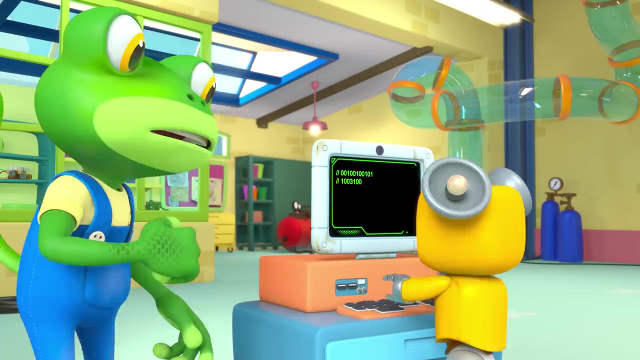 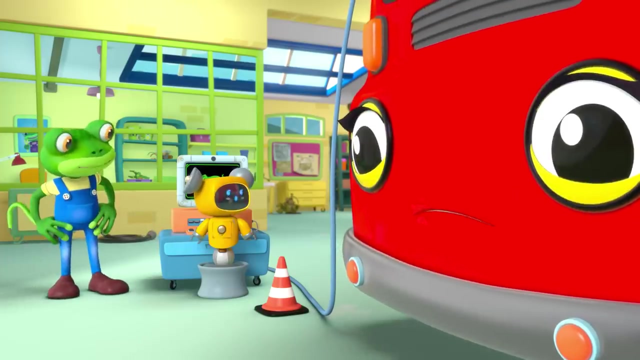 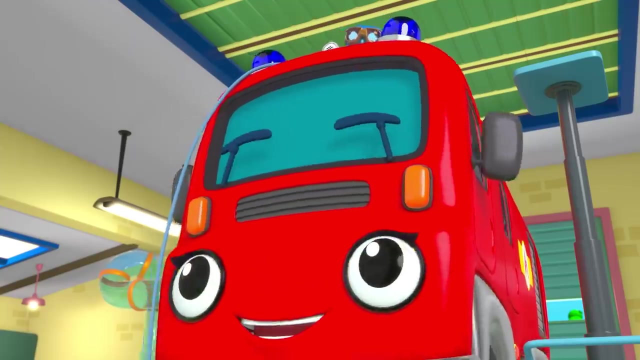 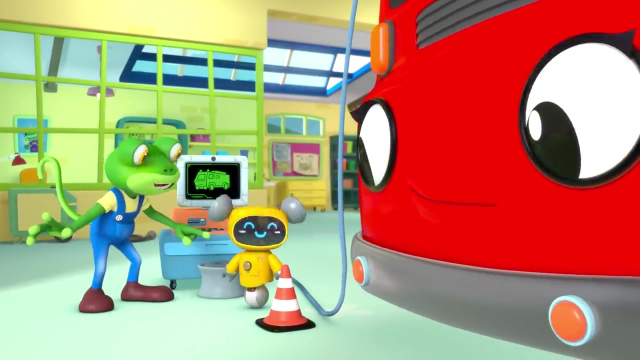 All done. Give it a go, Fiona, That's not right. It sounds like a doorbell. Let's try again. And that sounded like a dinosaur. We need a neenaw. That was a neenaw, But it needs to be much louder. Hmm, that traffic cone made you louder, Yellow. 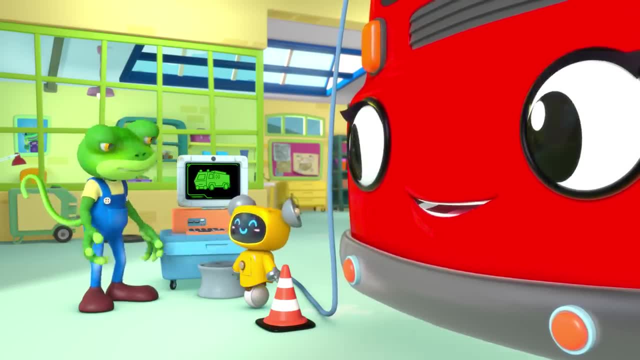 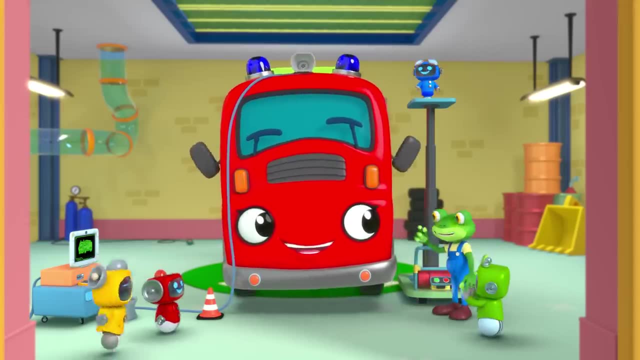 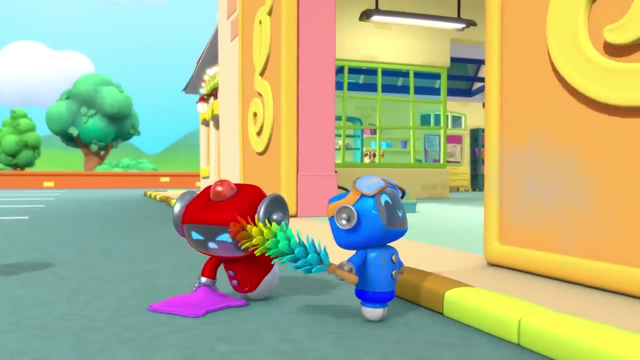 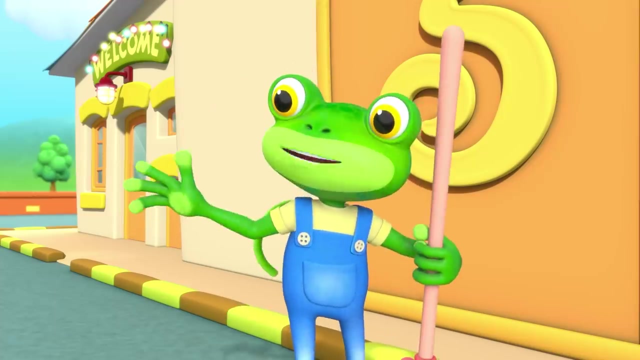 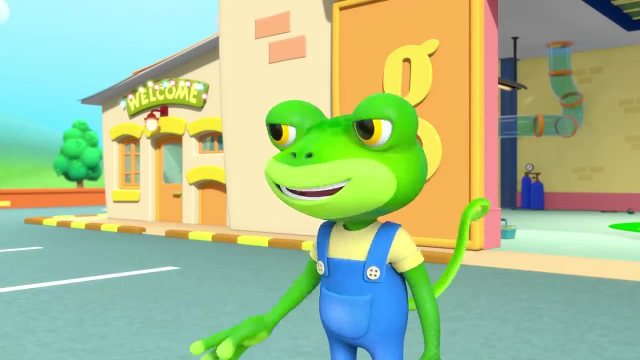 Maybe something like that will work with a siren. Now that's a loud neenaw. That's right, Mechanicals, Let's get the garage nice and clean. Oh, sounds like we've got a customer. It's the Truck. Family Mummy, Truck, Mama Recycle. 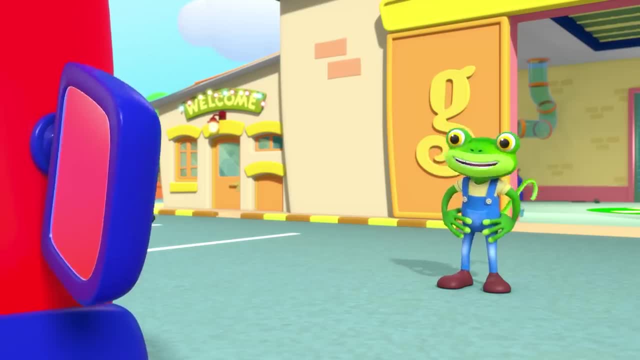 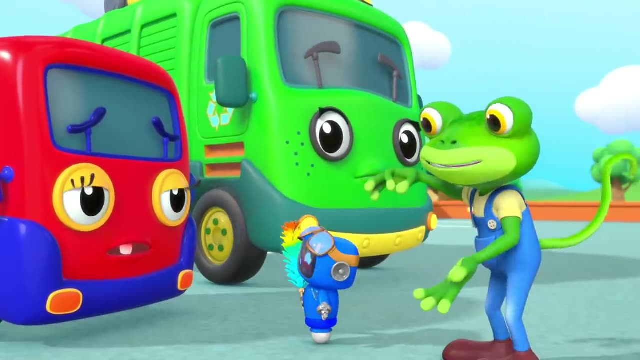 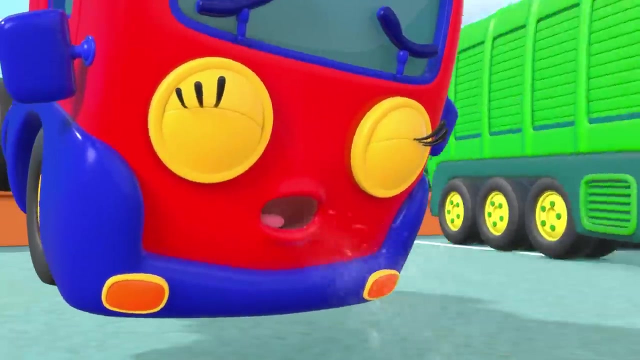 And Baby Truck, Who doesn't look very happy. A wobbly tooth, That's nothing to worry about, Baby Truck. When it falls out, you can place it under your pillow And you get a gold coin. Oh no, Baby Truck sneezed her wobbly tooth away. 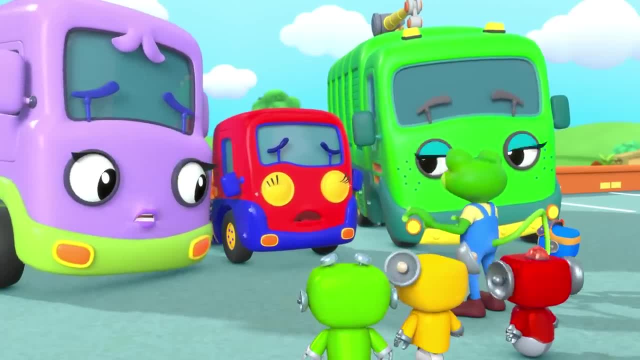 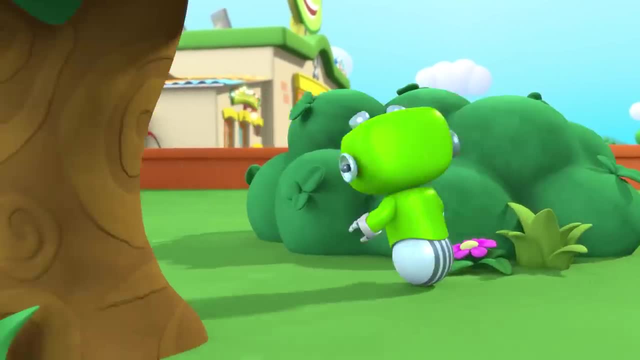 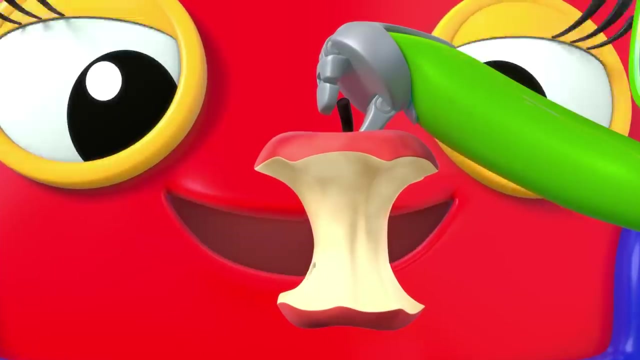 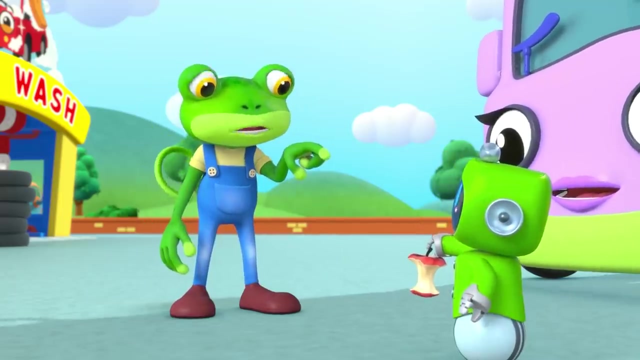 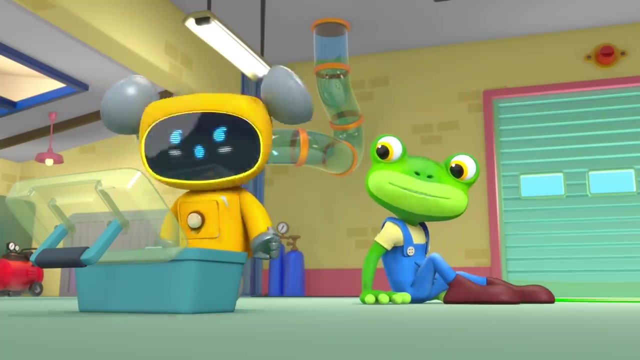 Oh, don't worry, we'll find it. Go go Mechanicals. Sorry Green, that's not a tooth. Oh gross, Sorry Green, that's not a tooth. Oh no, Let's just eat them. Oh Whoa, watch it Yellow, Oh no. 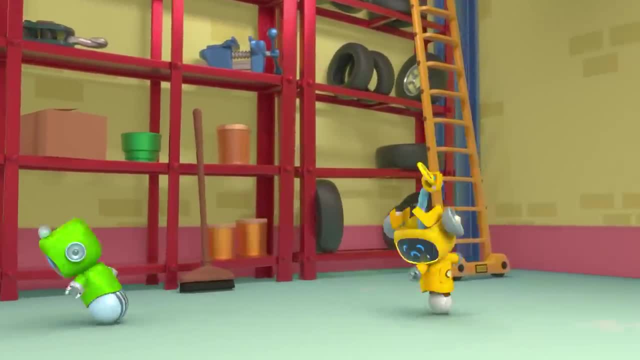 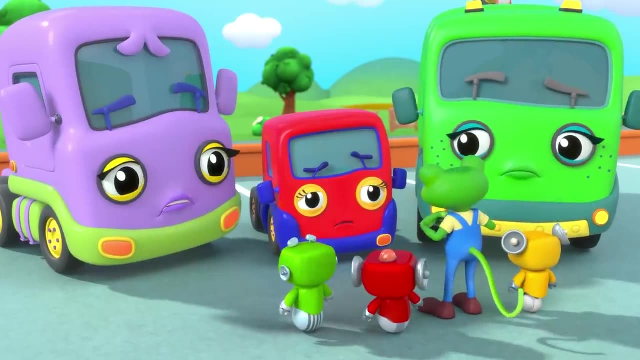 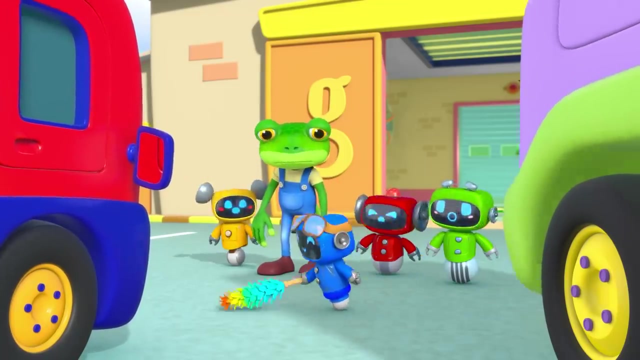 Please don't make that noise. Oh no, It can't be helped. Oh no, Oh. We've searched the whole garage and there's no sign of Baby Truck's tooth anywhere. Just a minute, there's one place we haven't looked In: Blue's Feather Duster. 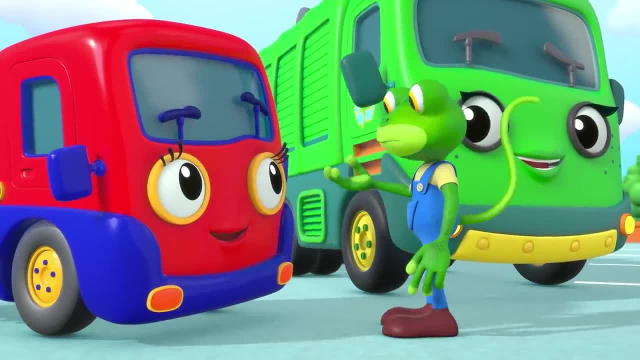 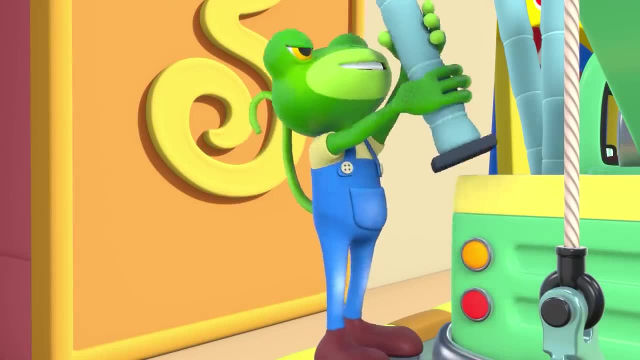 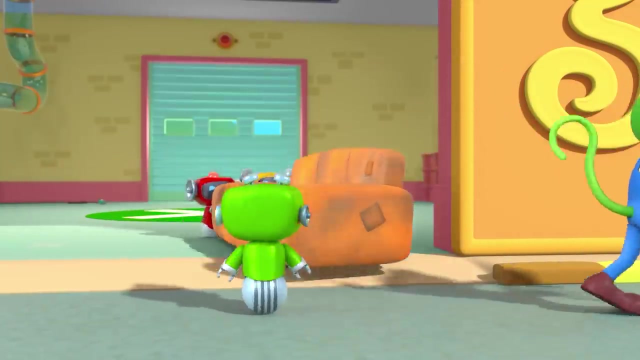 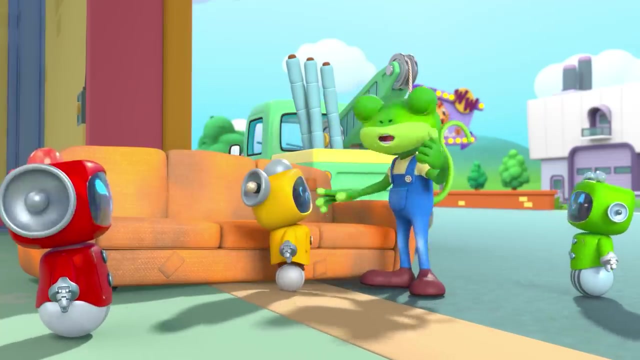 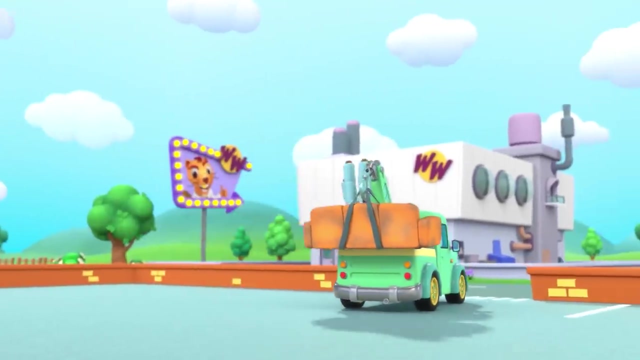 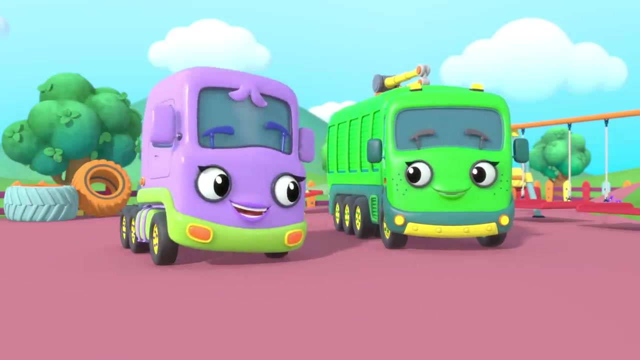 Here you go, Baby Truck. now get home and put it under your pillow. Come on, Green, let's load all this rubbish into Tilly Whoops. Sorry, Yellow, that old sofa needs to go to the rubbish dump. we can't keep it. It's the Tramp Family, Mummy Truck, Mama Recycle and Baby Truck. 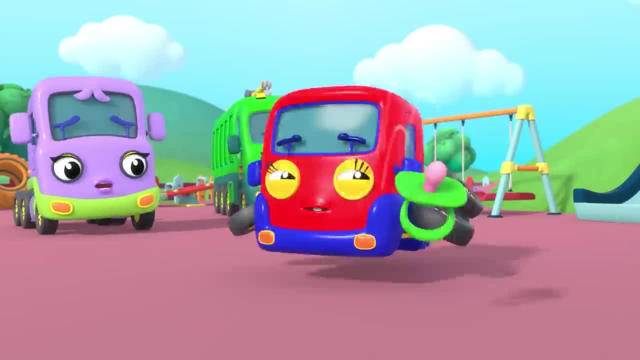 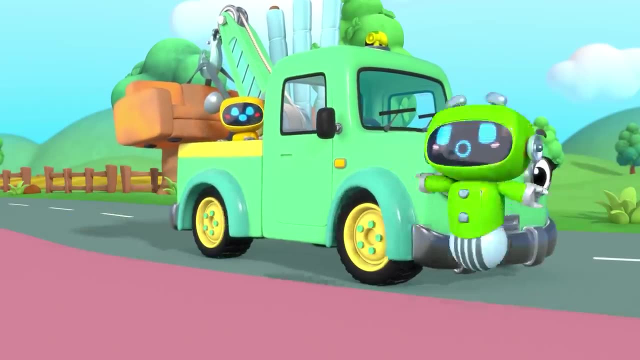 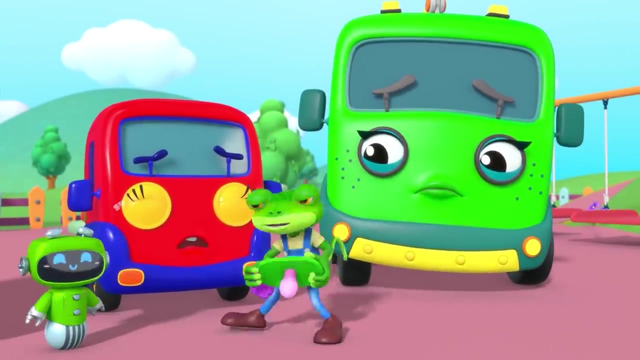 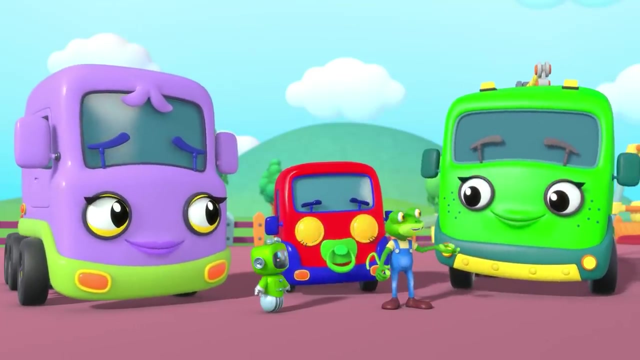 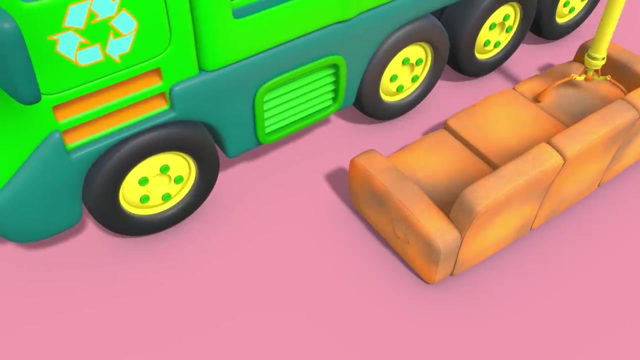 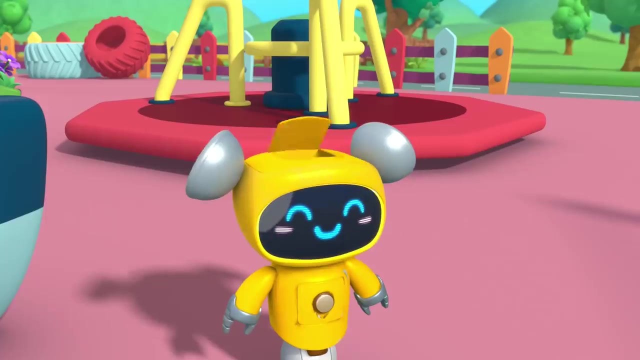 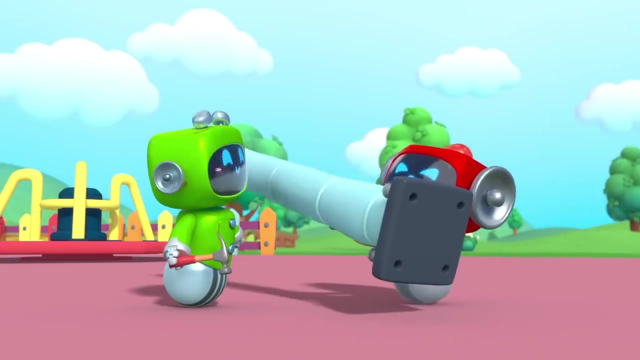 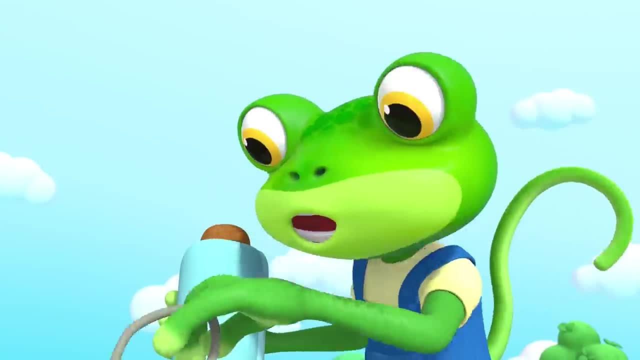 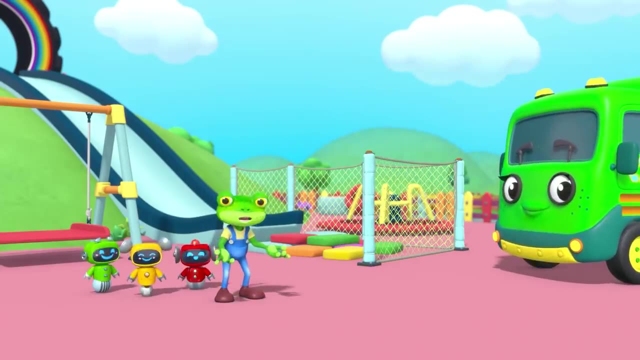 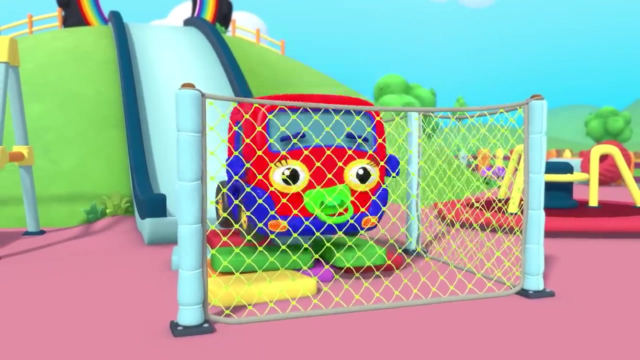 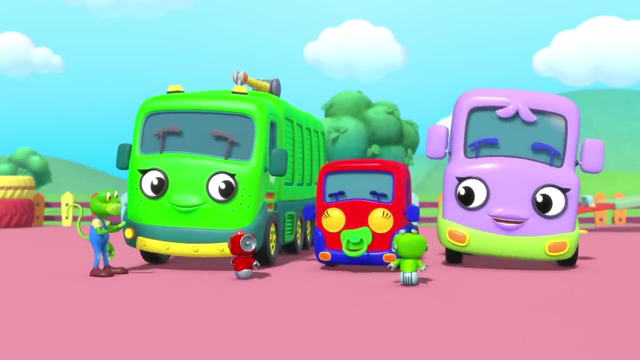 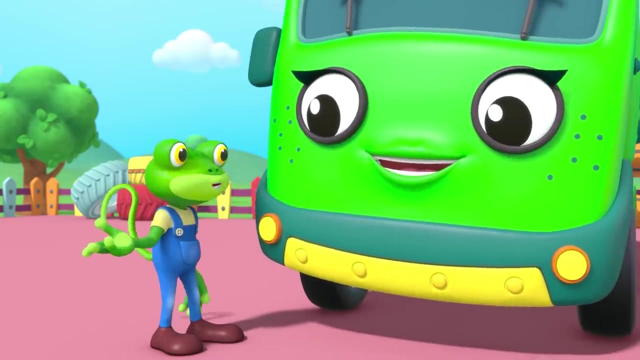 Shush, Shush, Shush, Shush, Shush, Ta-da, There you go, Baby Truck. You should land softly this time. You're welcome, Baby Truck. Aw, thanks, Mama Recycle. It's always good to make something new out of something old. 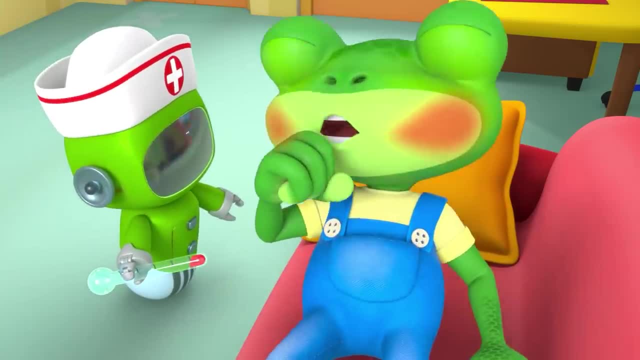 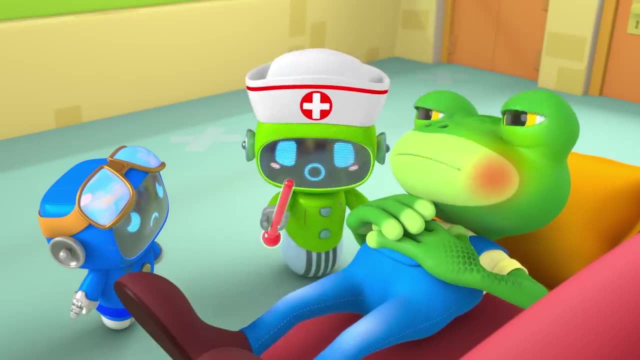 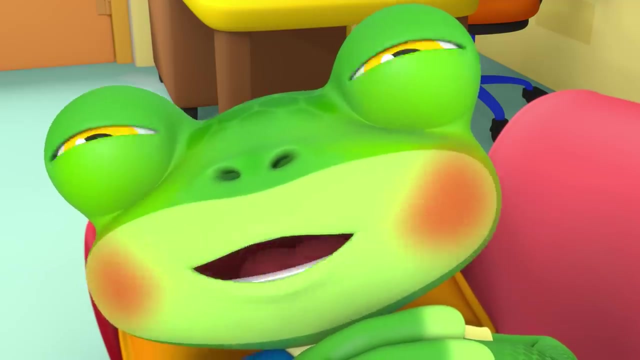 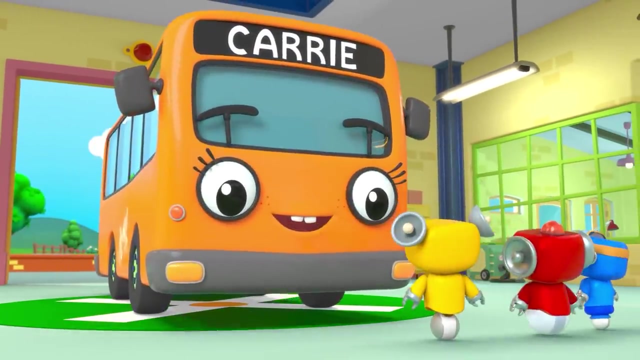 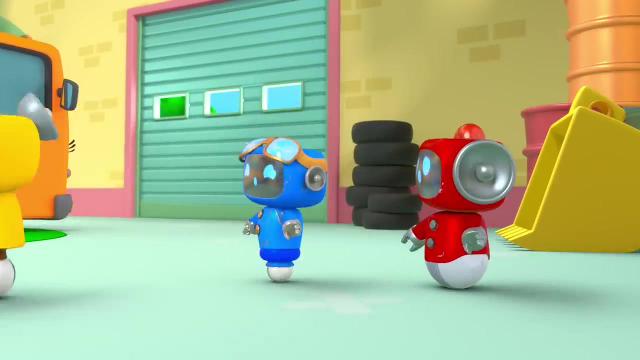 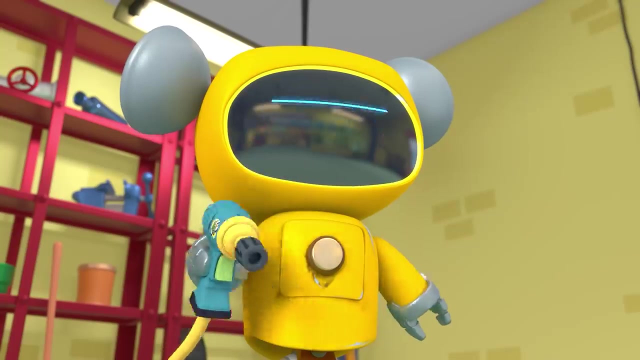 I don't feel so good. Oh dear, Oh dear, Oh dear. It's carried the busiest service today. Can you handle that, Mechanicals? Yeah, sure, Huh, Oh, Uh, Hm, Uh-oh. 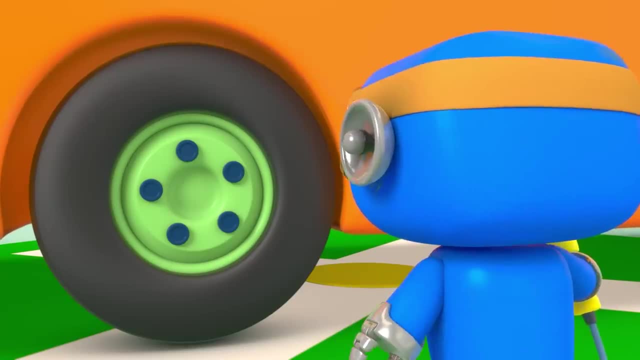 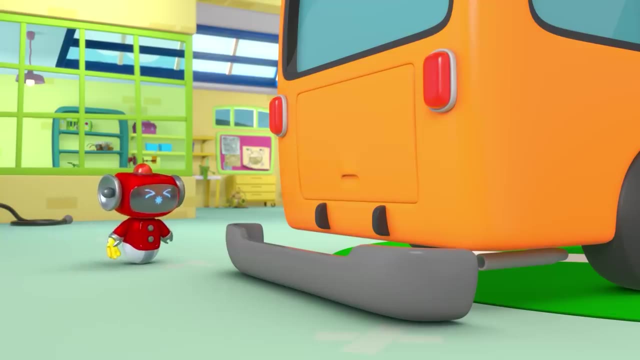 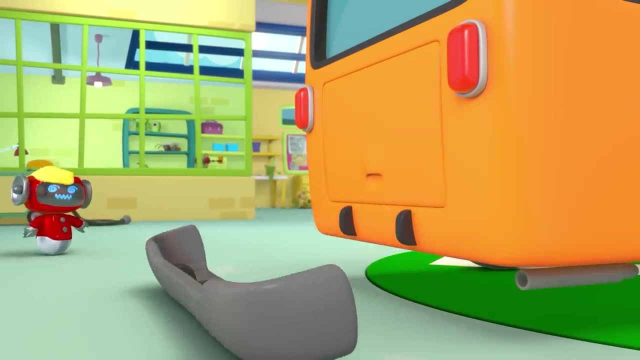 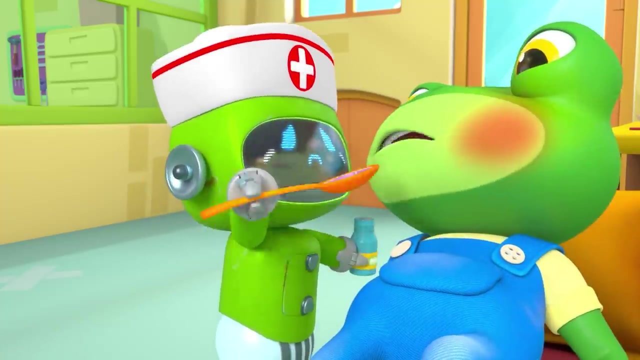 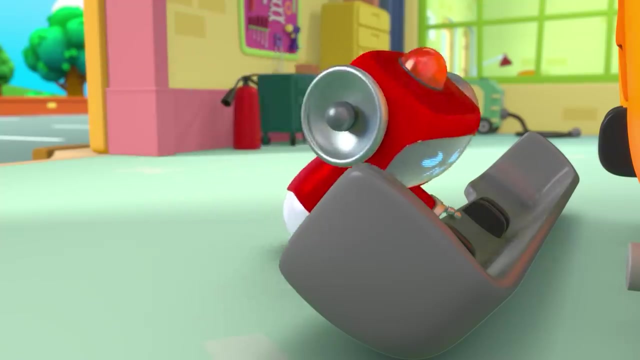 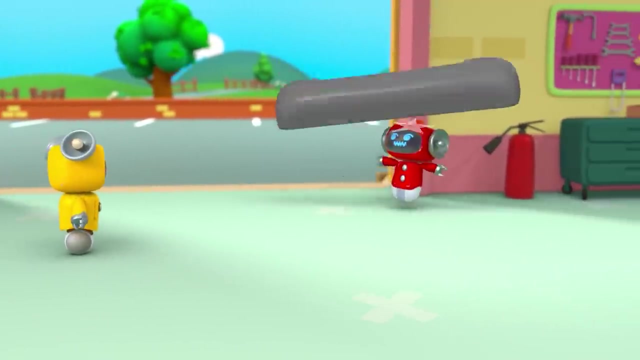 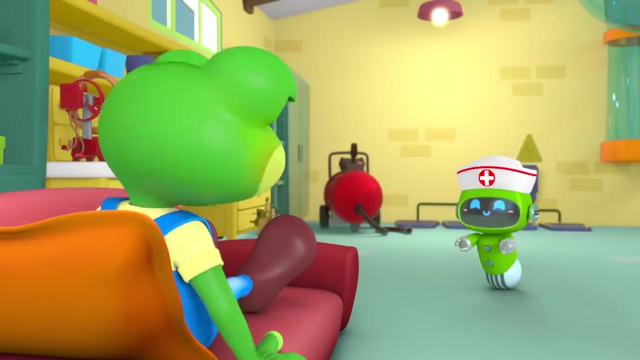 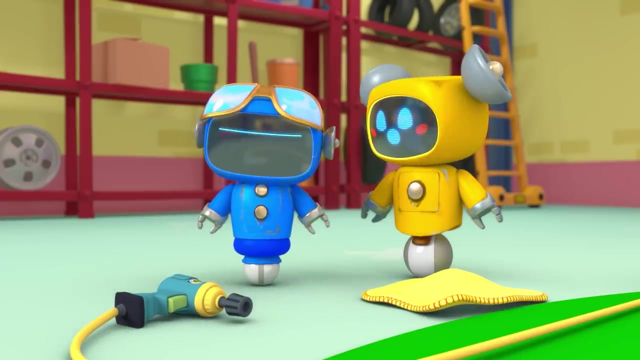 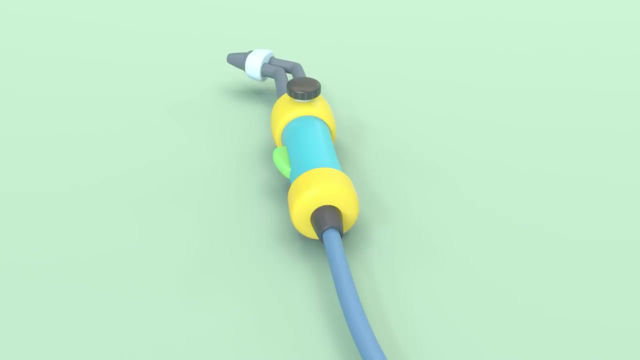 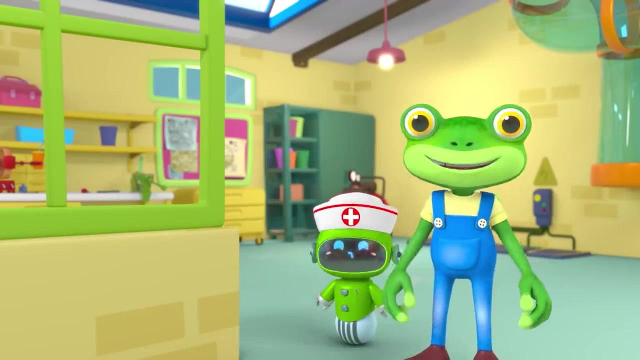 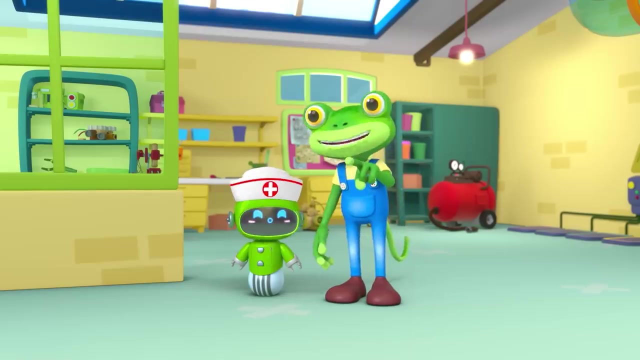 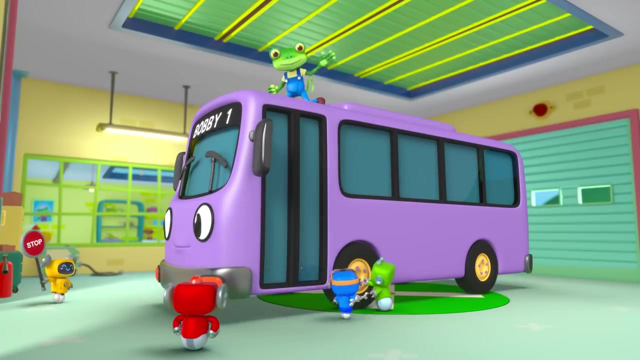 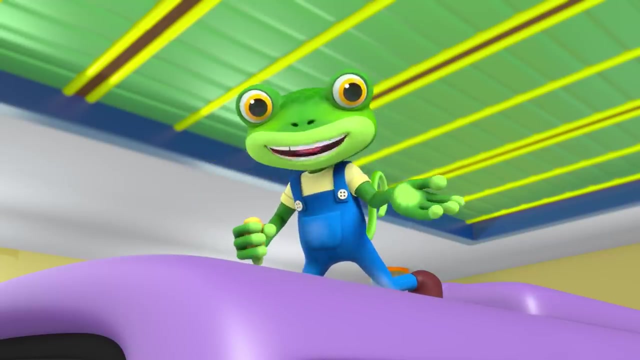 Hmm, Hmm, Oh, my goodness, Oh, dear Sorry. Oh, Is everything okay? I feel a bit better now. Looks like the mechanicals have it all under control. great job everyone. Hey, everyone, welcome back to geckos garage. We're just giving Bobby the bus his checkup. We're almost done. 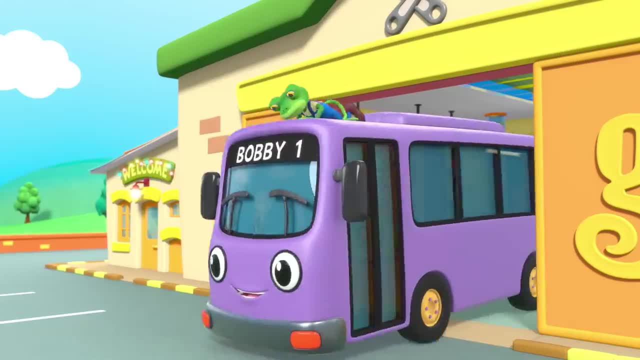 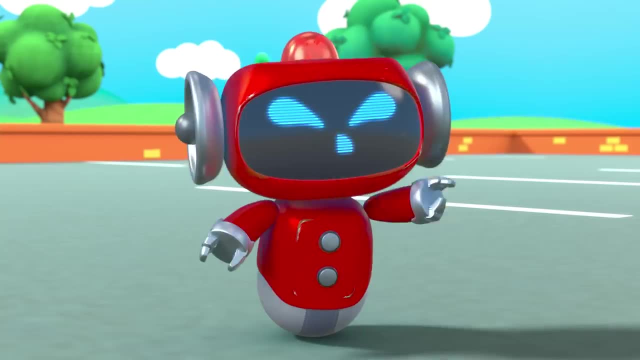 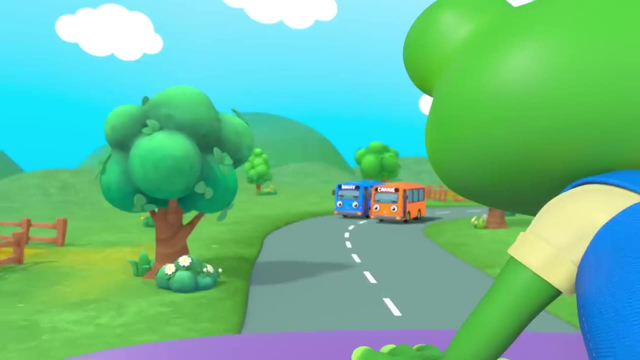 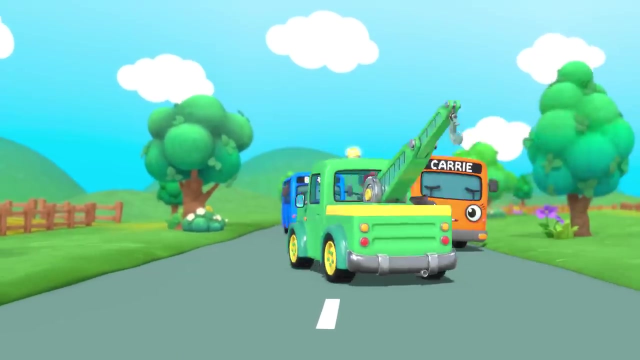 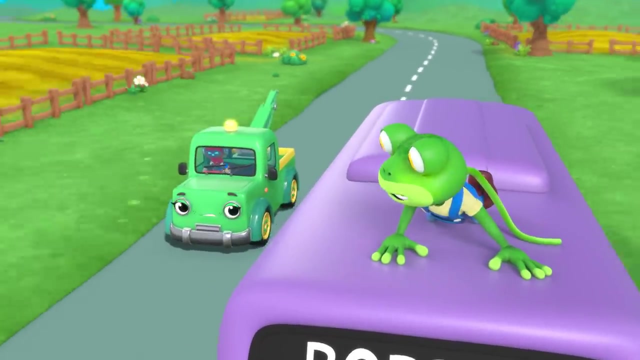 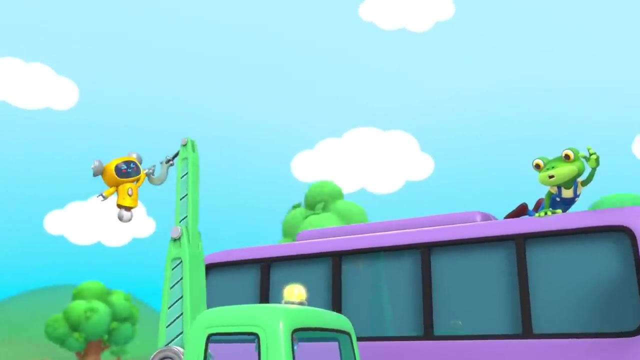 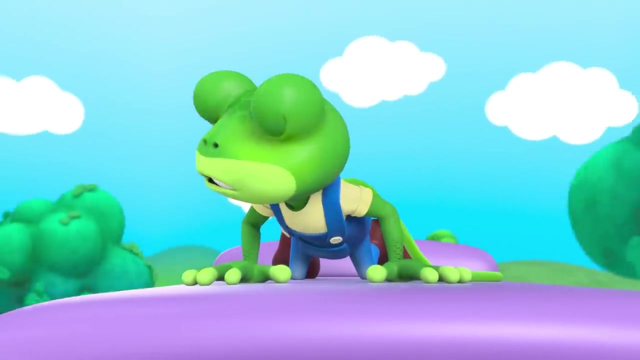 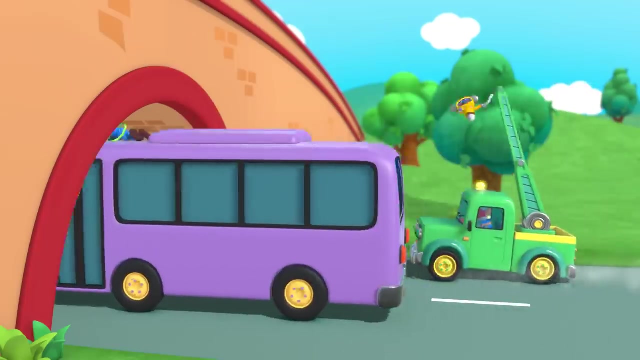 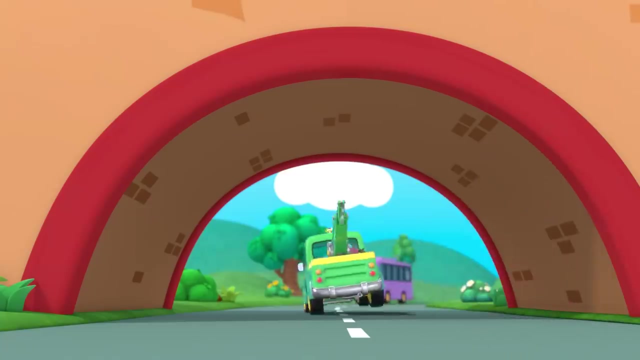 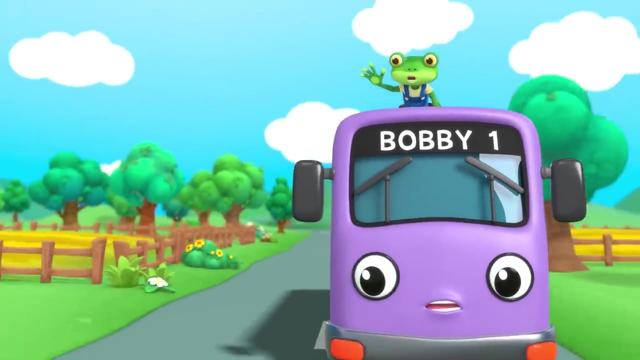 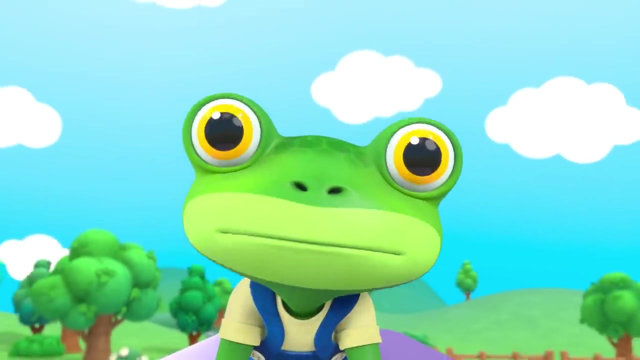 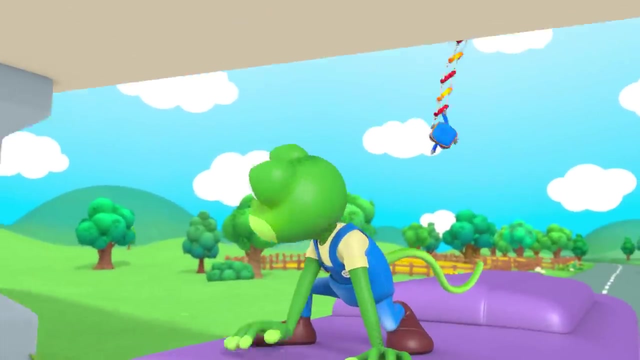 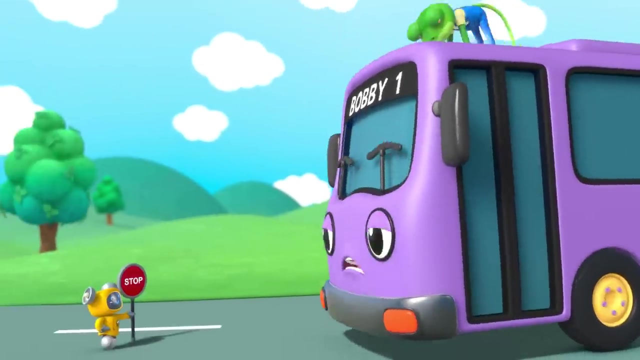 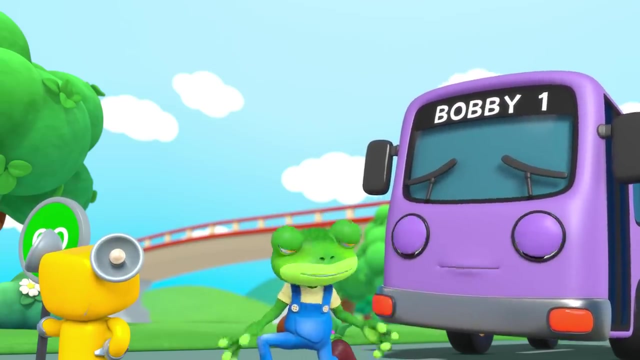 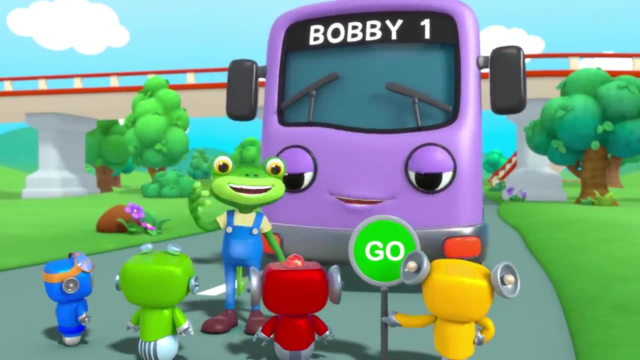 Oh dear, he can't hear me. Mechanicals, quick, do something. Here comes a bridge, Spinning screwdrivers. Oh Look, a high bridge. Great idea, mechanicals. if I can just wrap It up: Good thinking, yellow, you save the day. It's okay, Bobby, you didn't know and nobody got hurt. Thank you for all your help, mechanicals. 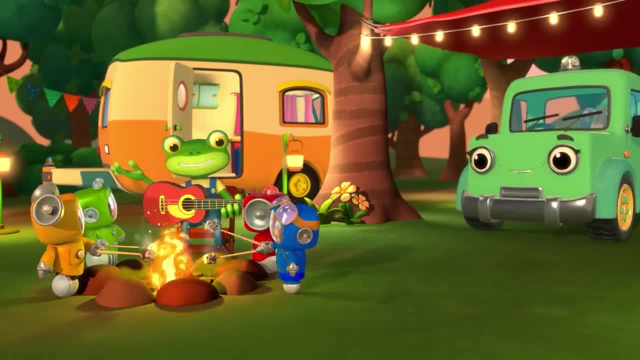 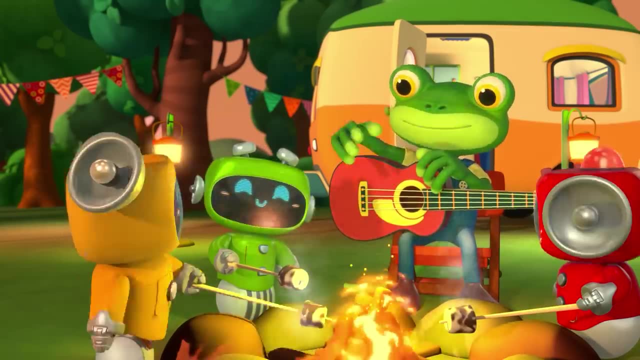 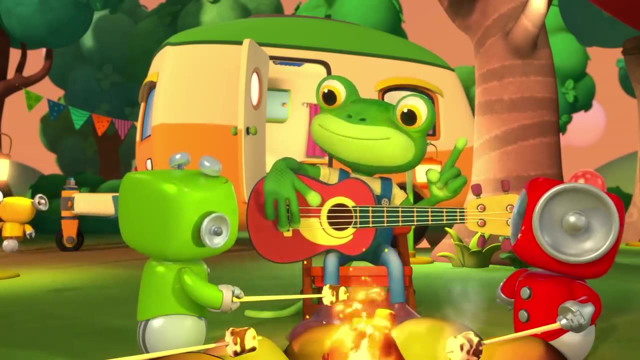 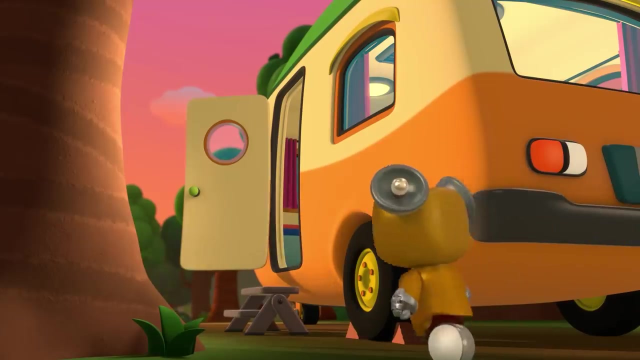 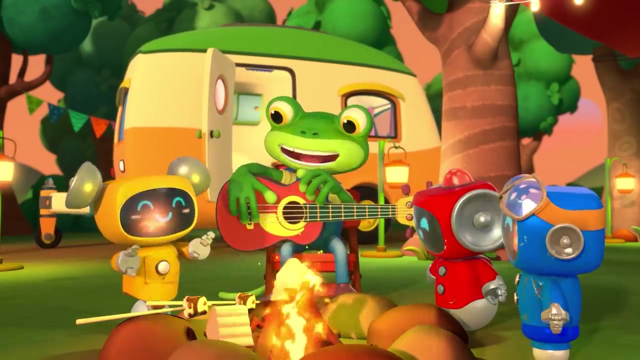 Ah, It's so nice to have a holiday. I love camping. Hmm, the fire's getting low yellow. Could you grab some more firewood please? Then it's time for a story. I think the storybook is in the caravan green. Thank you. yep, wait a moment. These are the wheel stops, which means 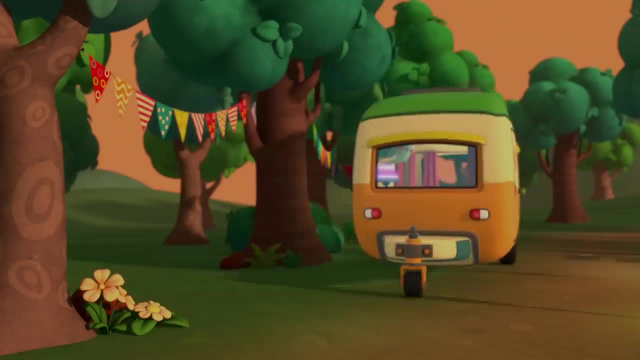 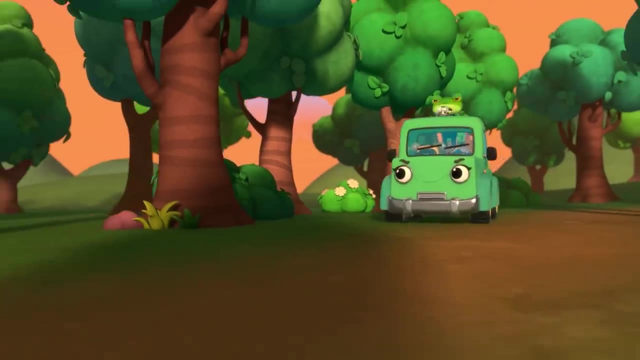 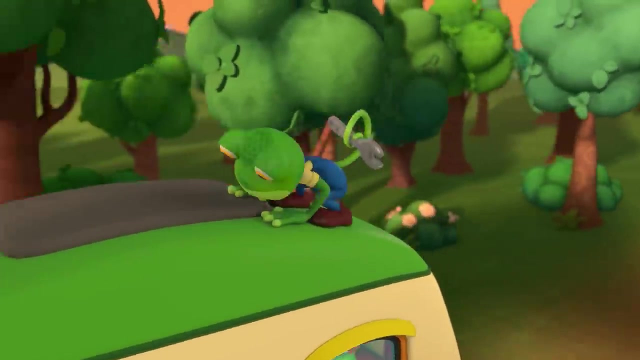 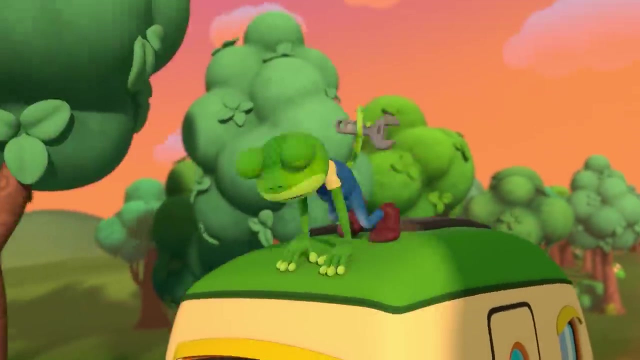 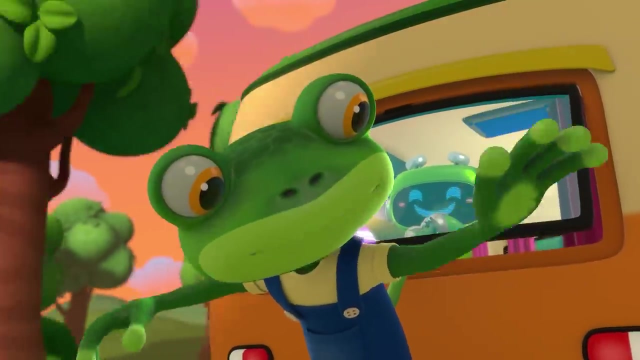 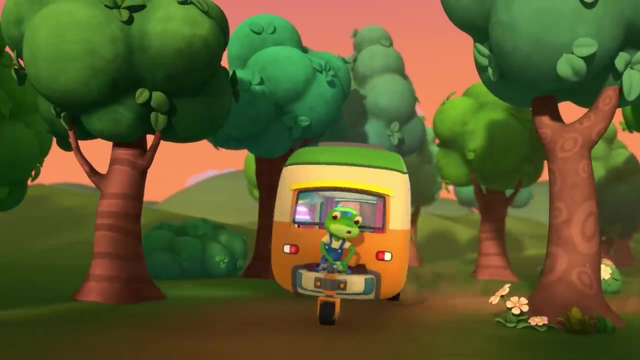 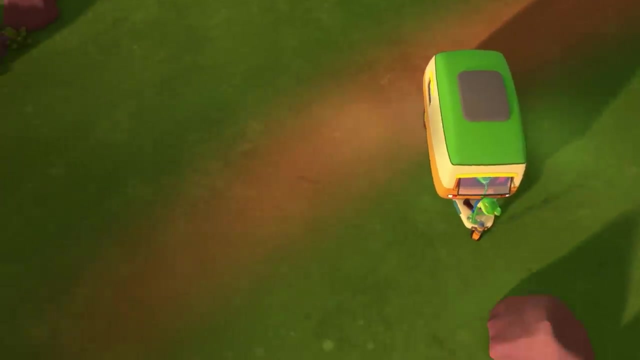 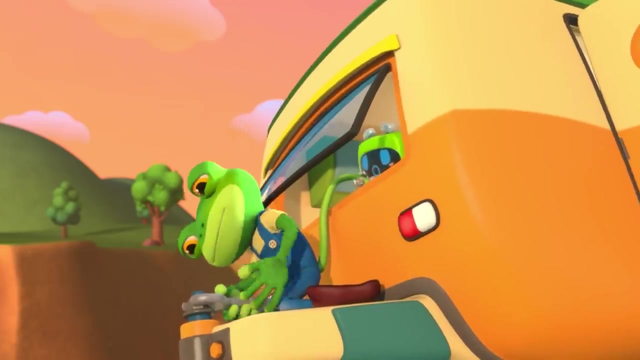 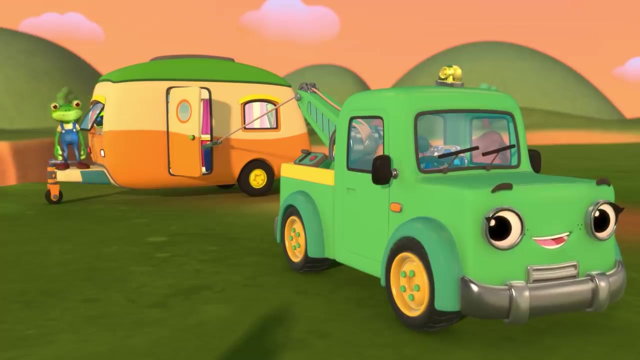 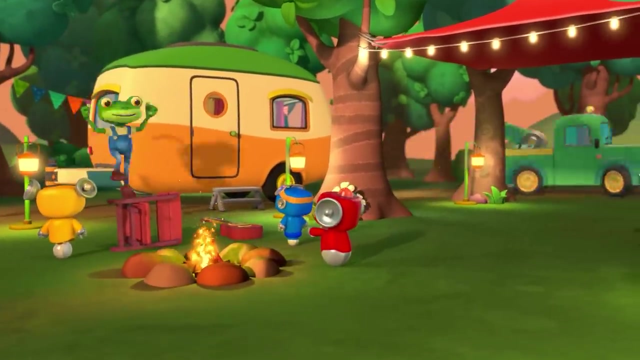 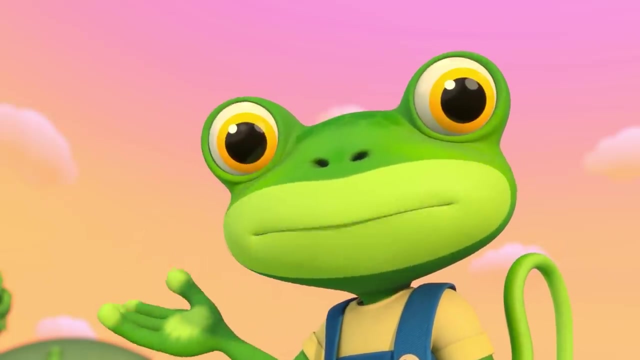 Quick catch that caravan. Oh, There must be a way to stop this. Oh Thanks, green. Spinning screwdrivers: Hooray, Nice work Tilly. Oh, good job everyone. Panic over. Yes, Green, It is story time now. 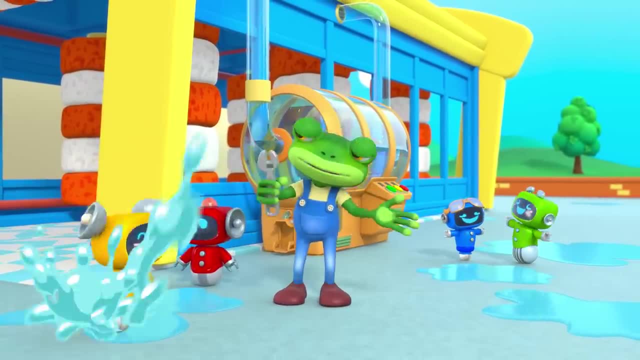 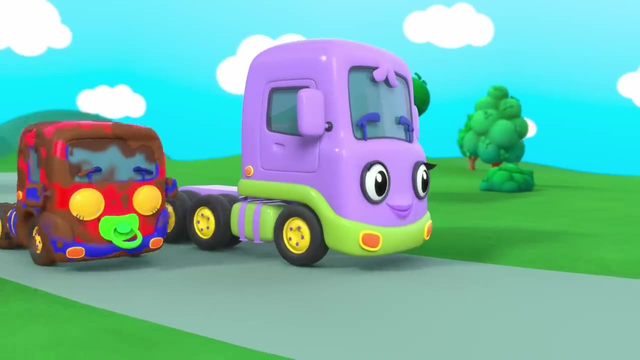 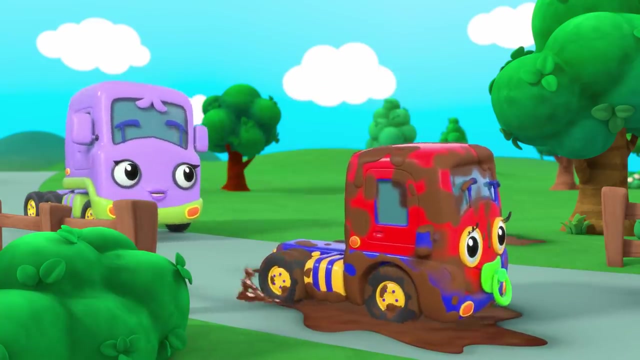 Hello everyone, Welcome back to Gecko's Garage. Oh, it's very muddy today, So we're getting our car wash ready. Oh look, Here comes Baby Truck to get all cleaned up. Ooh, Oh, hello, Baby Truck. 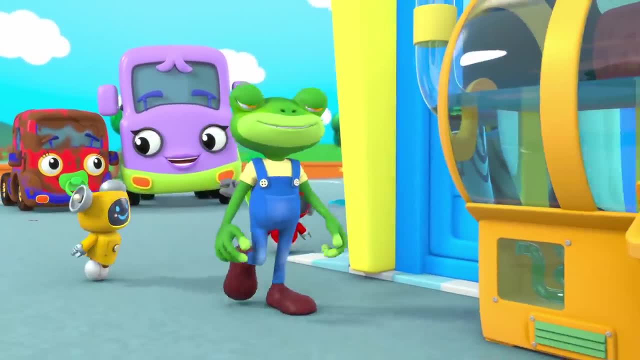 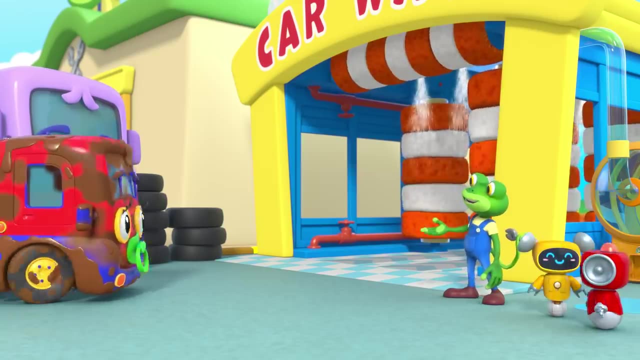 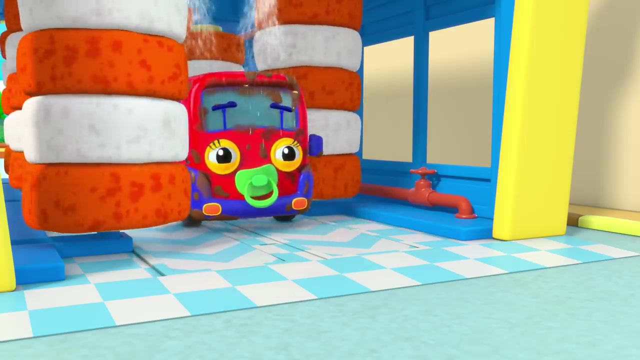 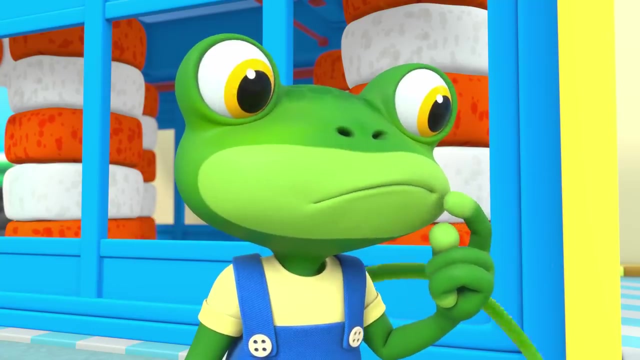 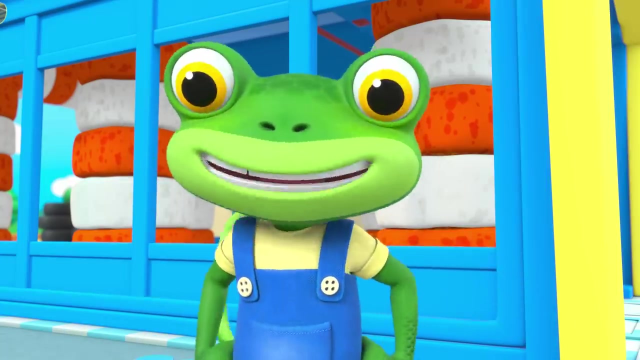 Let me guess what you're here for: Splish, splash and splosh Activate Gecko's car wash. Hmm, that's not right What? You're still all muddy. Of course We haven't filled it up with soap. 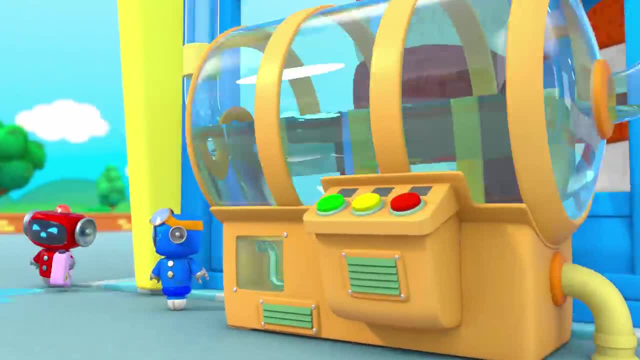 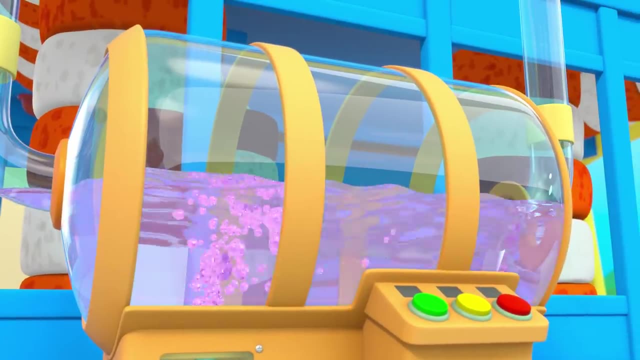 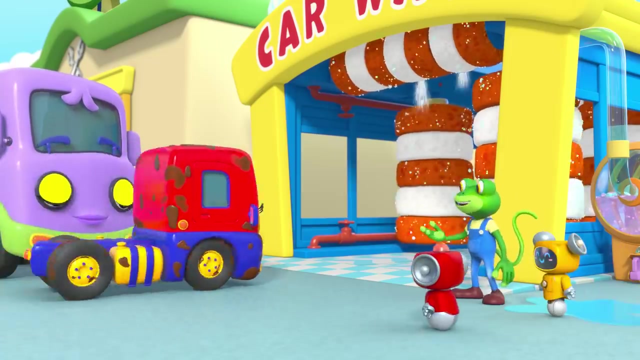 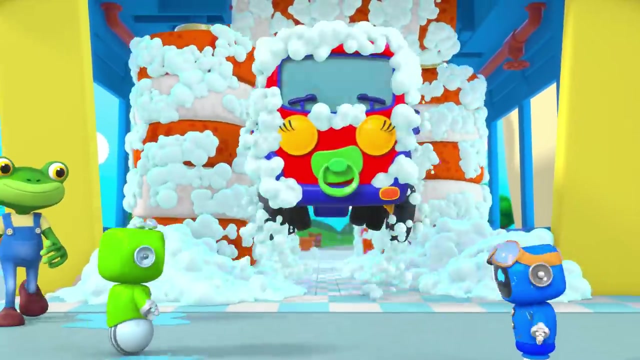 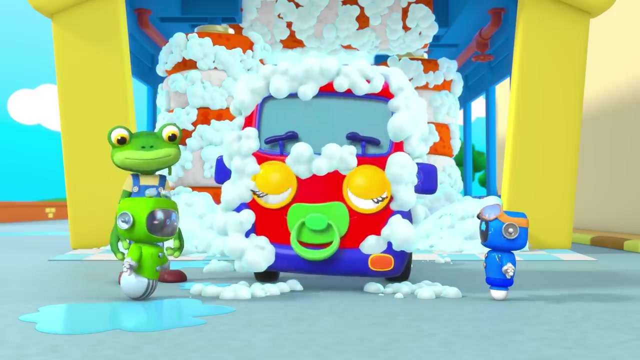 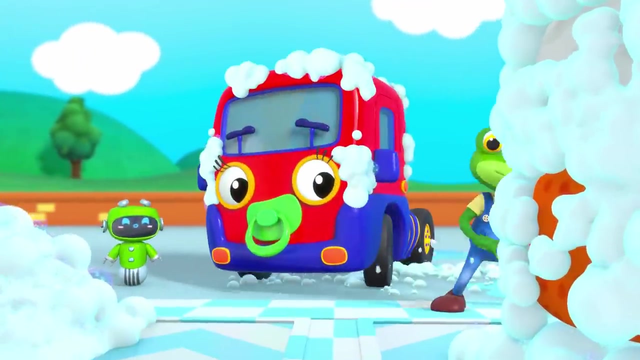 You can't get squeaky clean without soap. Now the soap is filled to the top, We can wash all that mud off. Oh, that's strange. The rollers are meant to roll the bubbles off. Hooray, Ooh, Aha, That's it. 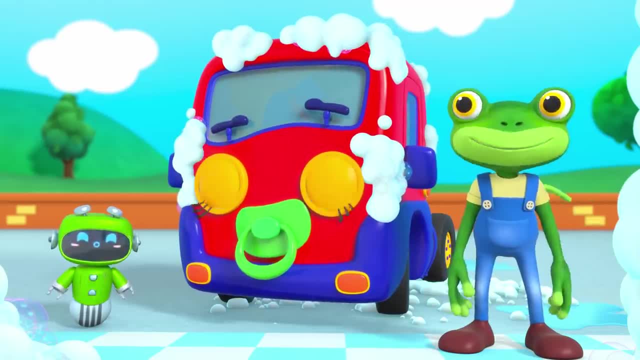 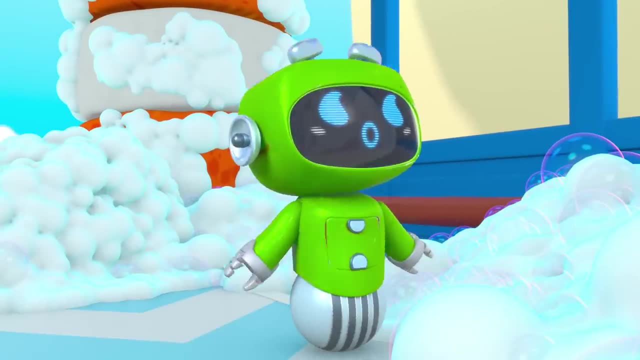 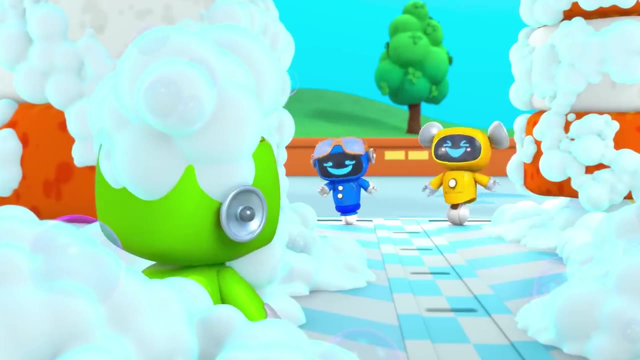 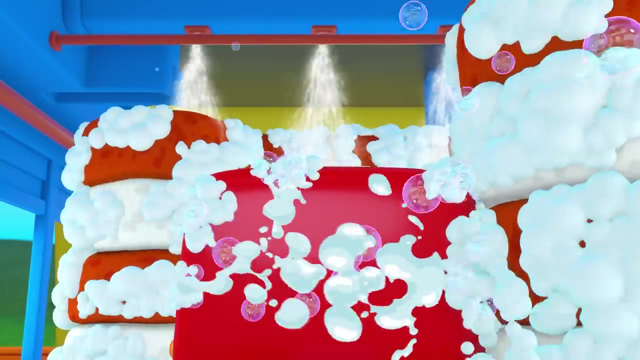 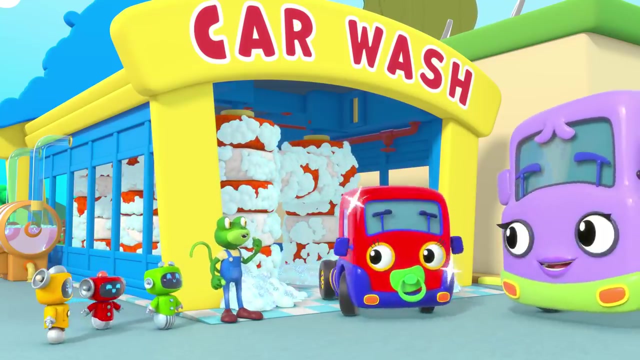 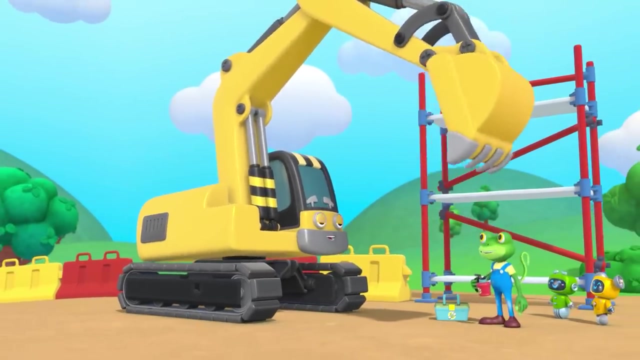 Baby Truck is too small for the rollers to reach. Ah, He-he Hooray, The car wash is working And Baby Truck is sparkling clean. Do-do-do-do-do, Ha-ha. There you go, Eric. All better now. 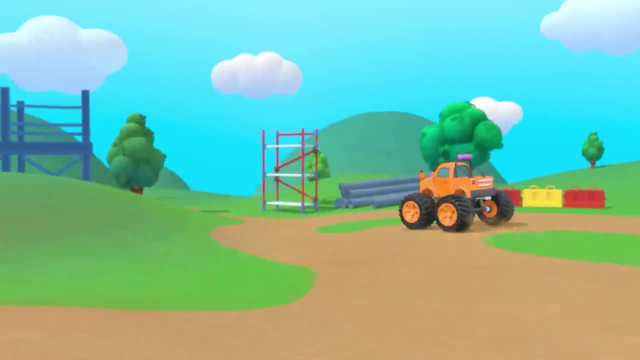 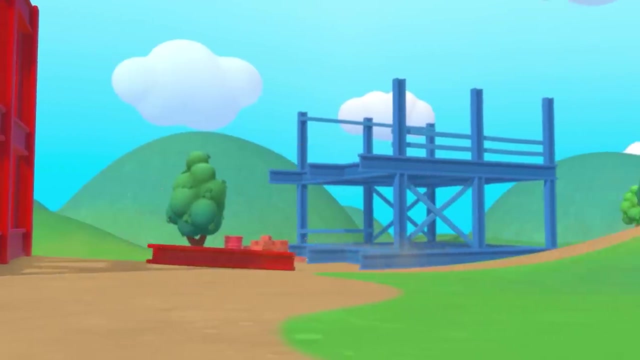 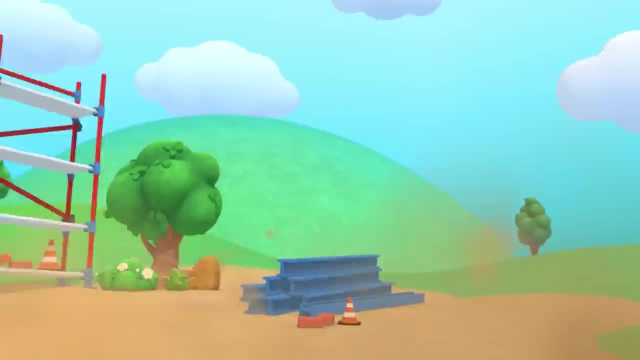 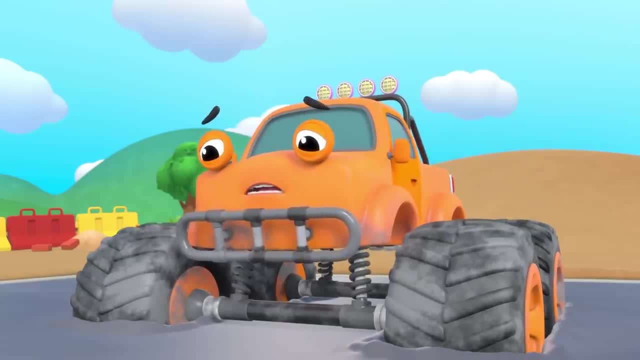 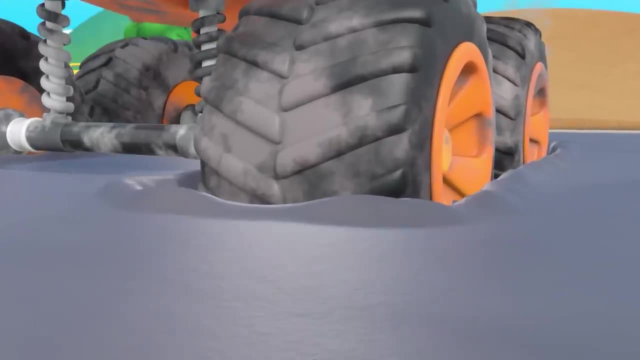 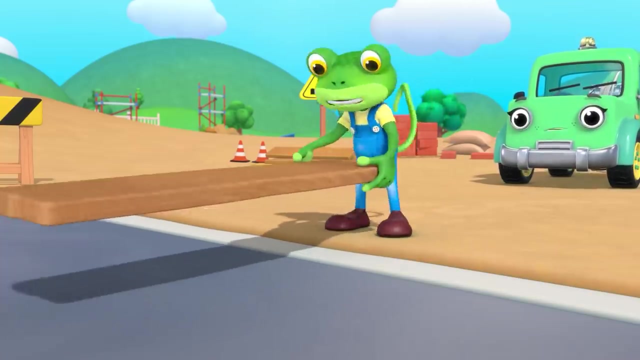 Ha-ha. Oh no, Max has run out of fuel. We've got to get him out before that concrete dries. Quick mechanicals: Fetch the spare fuel. Oh dear, That concrete will be hard in less than a minute. 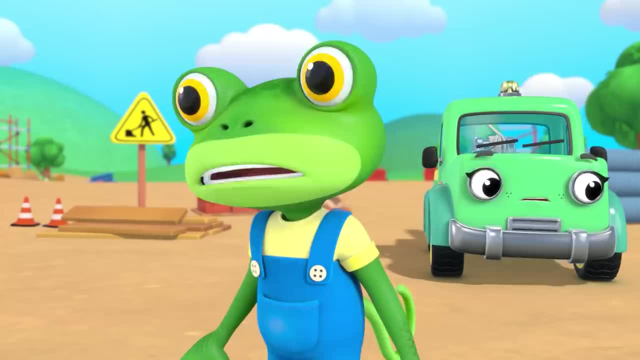 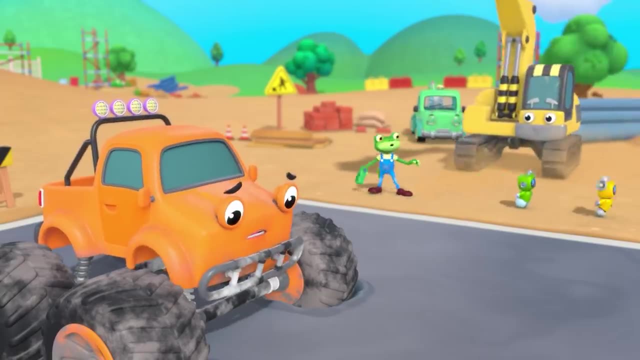 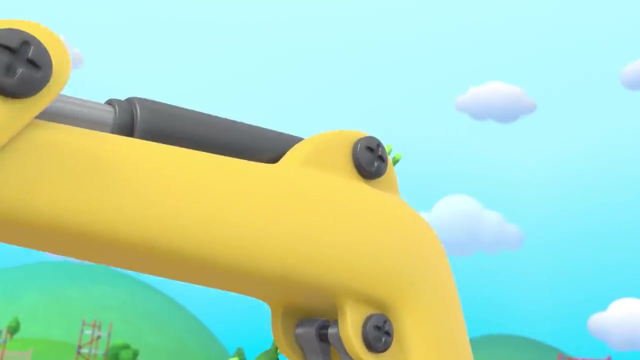 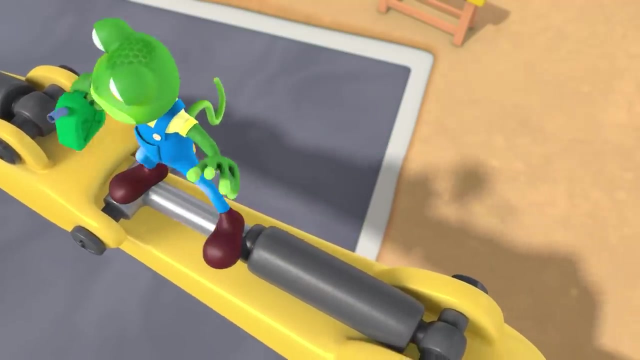 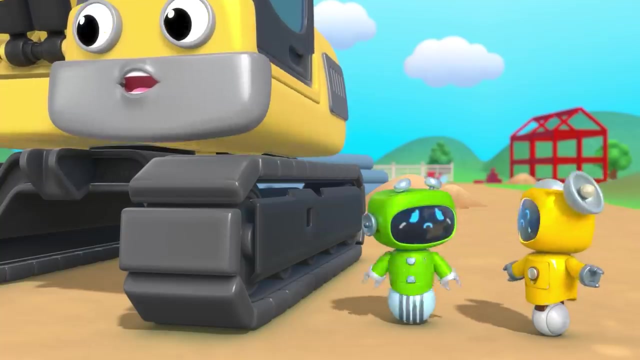 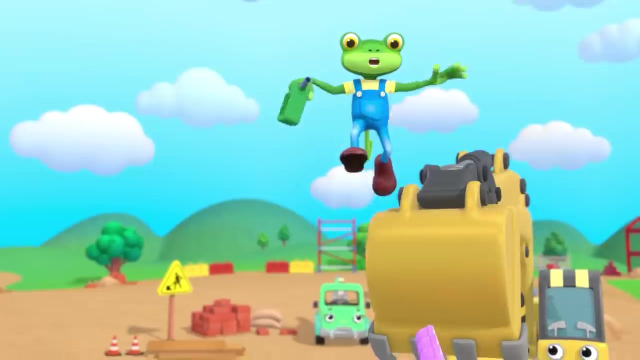 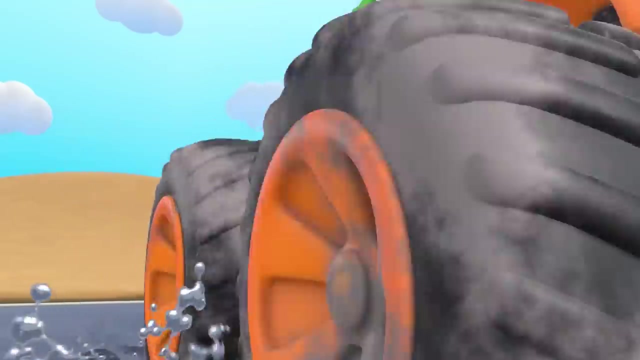 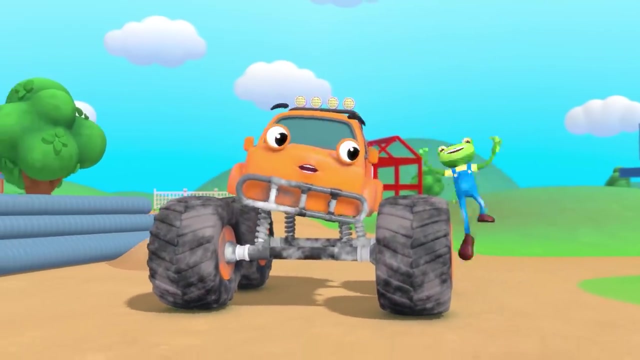 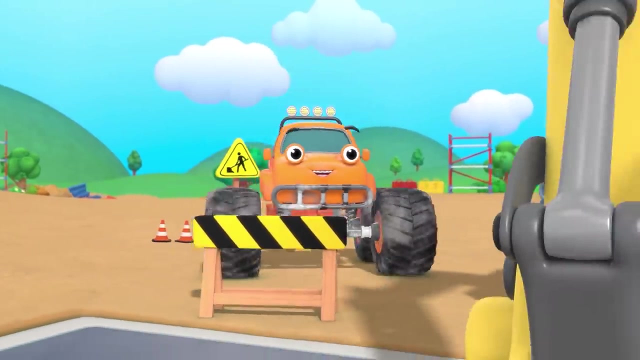 Oh, How on earth are we going to get the extra fuel over to Max? Eric's made a breach. Whoa, The concrete's almost set. Go, Max, go. Looks like Max has learned his lesson. Thanks, Max. Another panic over. 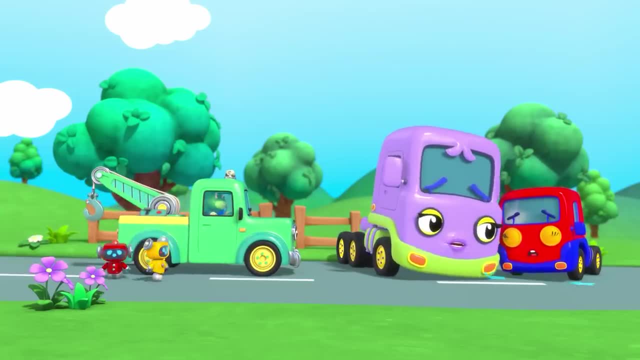 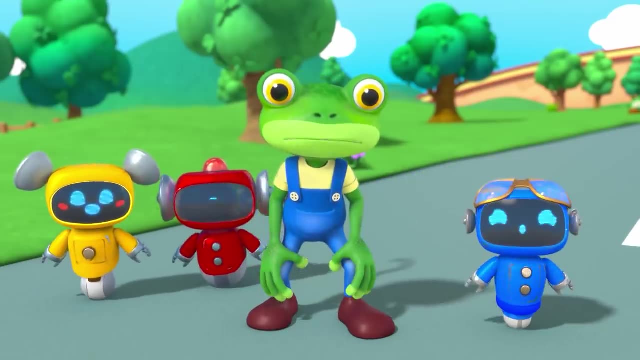 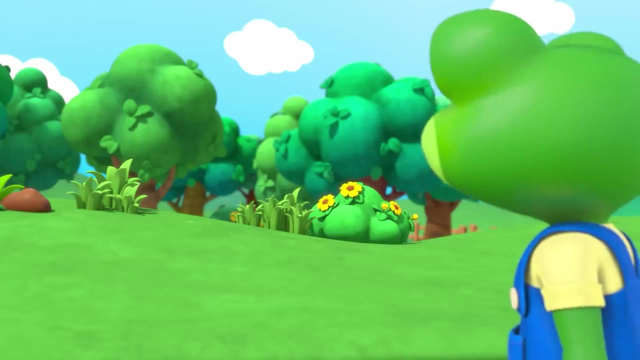 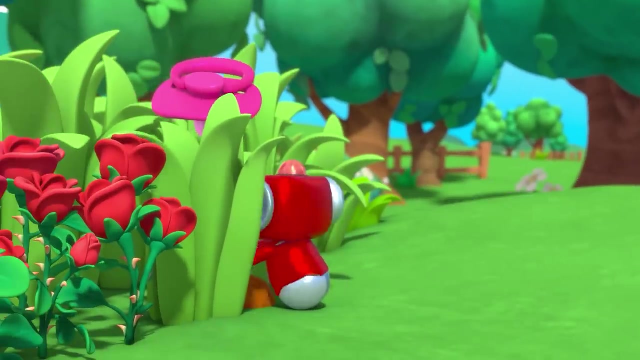 What It's Baby Truck? What's that Baby Truck? You've lost your dummy. Don't be upset, We'll find it for you. Go go Mechanicals, Go go Mechanicals. Try looking by those red flowers. 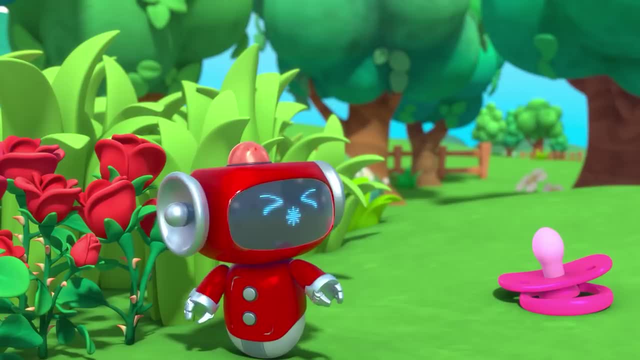 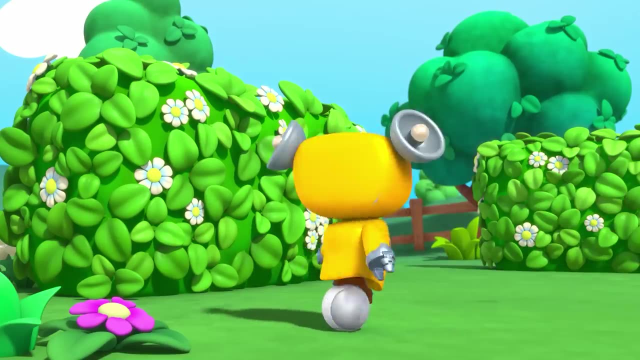 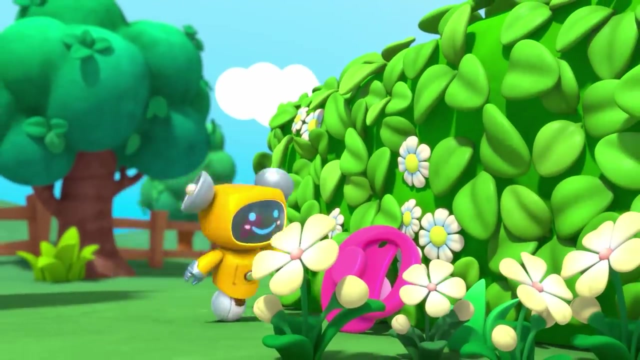 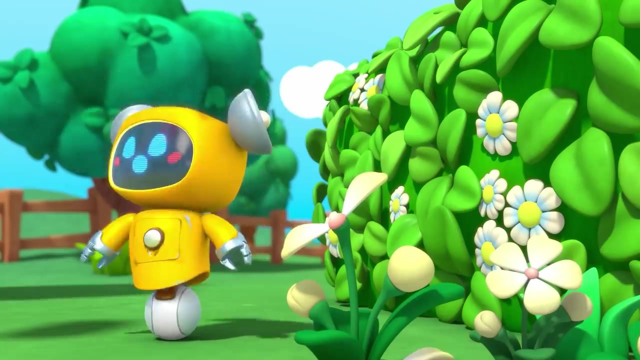 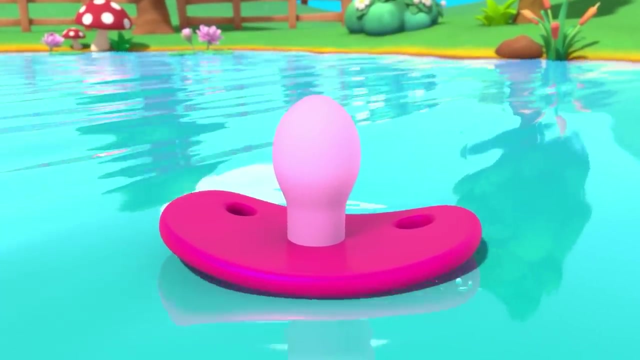 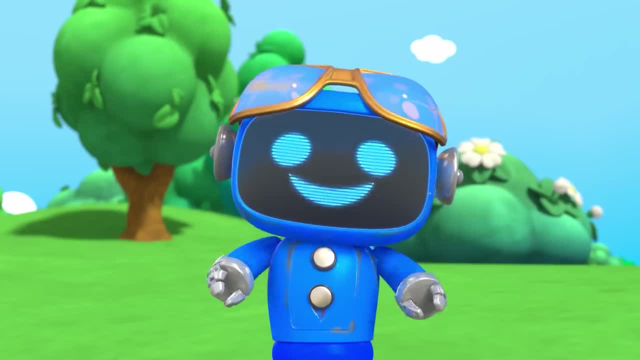 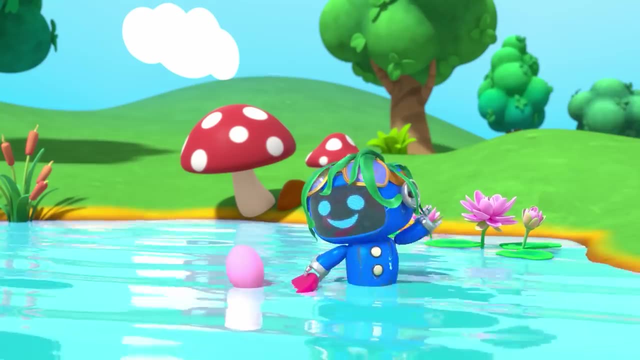 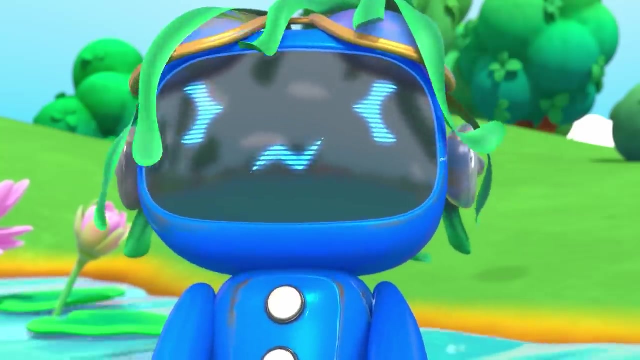